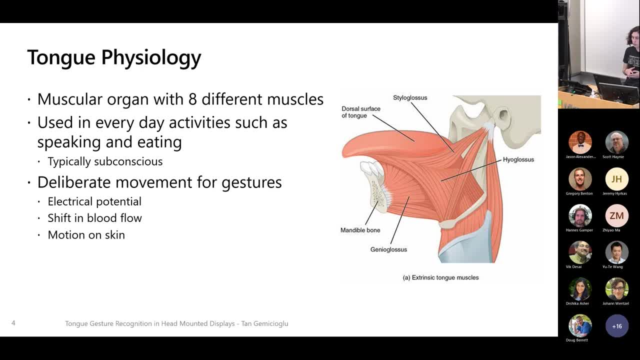 also make more deliberate movements, which is what we use for gesture interfaces, And it turns out, with the tongue these actually produce really, Yeah, visible signals, such as electrical potential that can be detected from above the skin, shifting blood flow around the face and you can actually also detect the motion. 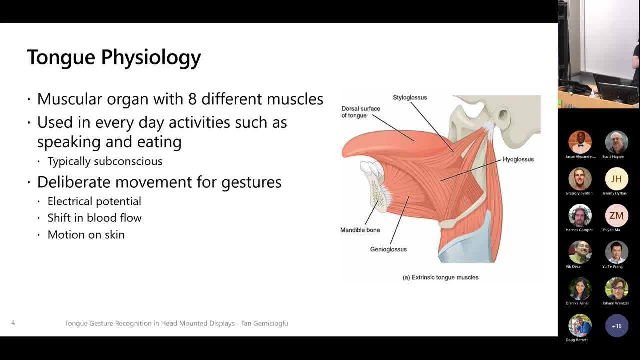 on the skin if you put your fingers at the back of your ears and try moving your tongue around a bit. And this is actually due to a muscle called the styloglossus, which goes from your tongue all the way up to the back of your ear. 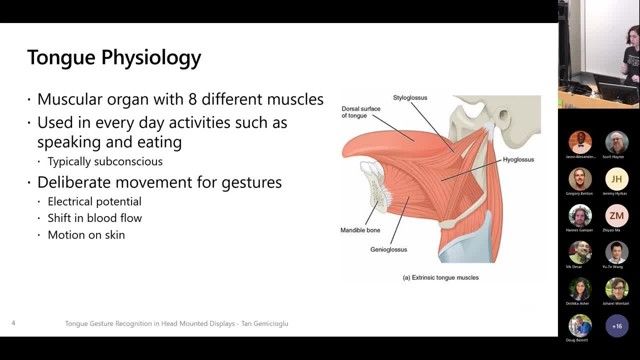 Okay, So this is actually a muscle called the styloglossus, which goes from your tongue all the way up to the back of your ear. Okay, So this is actually a muscle called the styloglossus, which goes from your tongue all the way up. 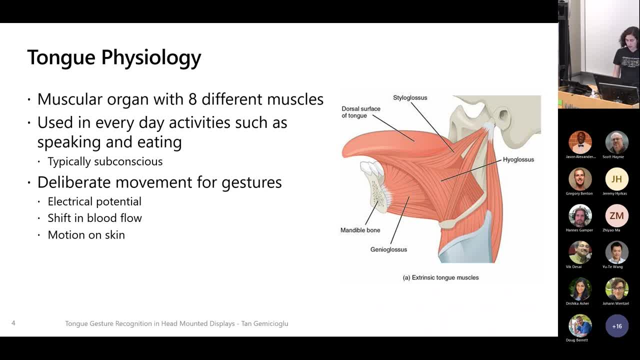 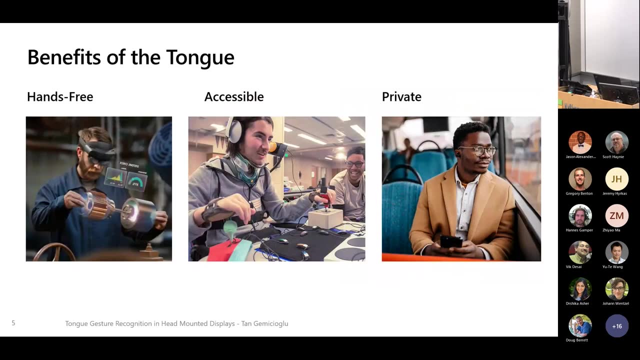 to the back of your ear and the top of your jaw And we plan the project to be able to use these signals and detect the tongue movements without necessarily being close to the tongue in our sensors- And the benefits of the tongue are actually quite a bit- that are useful in. 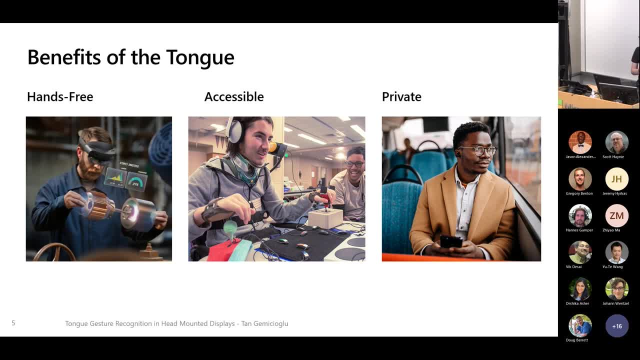 head-mounted displays. First off, it's hands-free, which is very relevant to many augmented reality use cases where people's hands might be busy or they might otherwise be unable to move it due to being in a crowded space. They're also accessible For people with movement impairments. 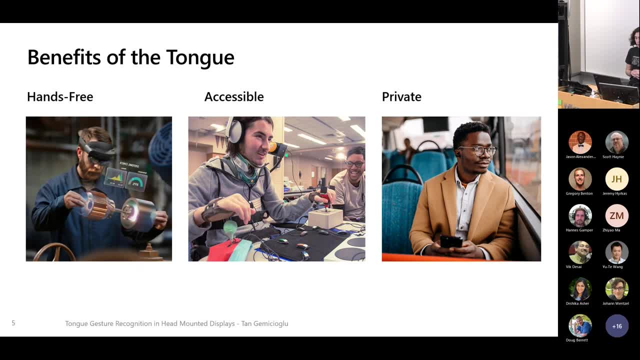 they might not be able to move their hands or use any other interface due to ALS, muscle dystrophy or similar muscle impairments. tongue interfaces often provide an alternative option, using the muscles that they have available for their movements. Tongue gestures are also private. 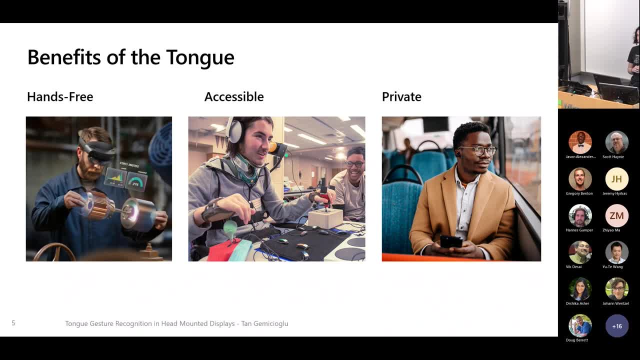 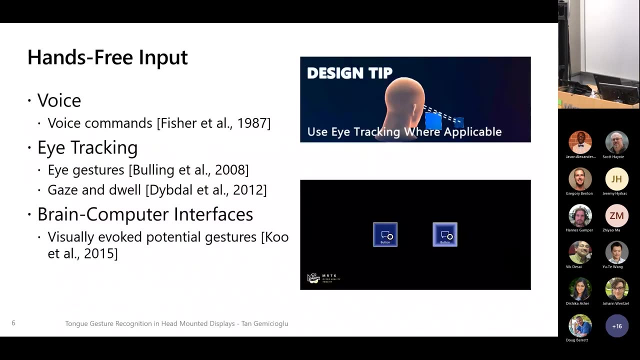 because any gestures that you do within your mouse are not visible to anyone and often also silent, which, compared to many other hands-free interaction methods, provides a big advantage. And with that mentioned, let's go into some of the other methods that are common in practice today. 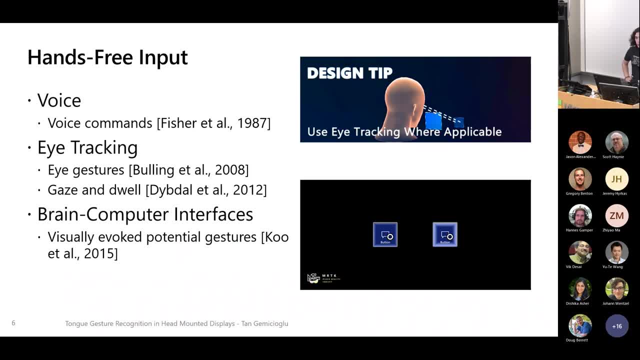 Since the start of head-mounted displays, voice commands have played an important part in being able to interact with head-mounted displays And, more recently, eye tracking has provided a silent option that is usable in a much wider range of environments. These started with eye gestures. 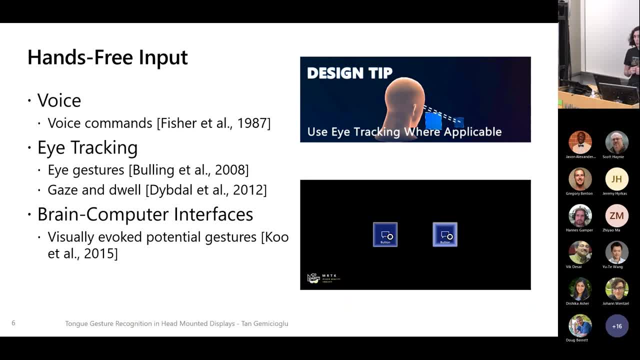 and then what's called gaze and dwell, where you look at a point and then focus on it to be able to trigger a response from looking there, And actually common in many applications using Microsoft Mixed Reality Tools and HoloLens And, even more recently, with brain computer interfaces. 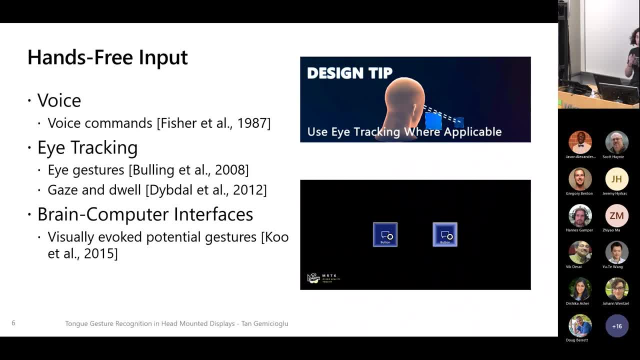 using visually evoked potentials, which are signals generated when you are looking at a particular point. we've been able to detect this from the brain as well, But both eye-tracking and brain-computer interfaces still require constant attention, which is not suitable in all cases. 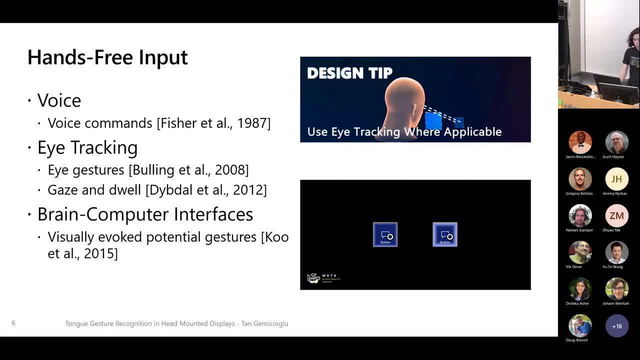 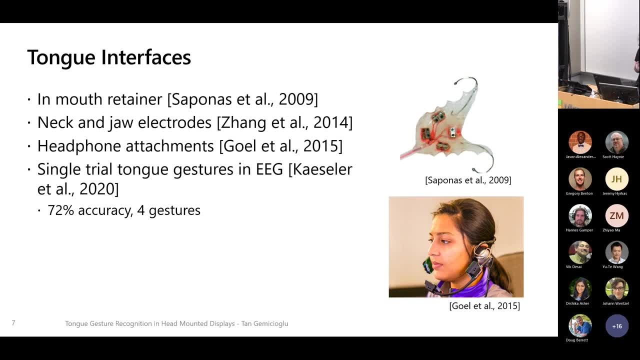 and they are also limited by their speed. Instead, tongue interfaces provide an alternative that is potentially faster and also does not require as much attention. This started actually here at Microsoft Research with in-mouth retainers by Soponis et al. These similar intrusive methods were the standard for a while. 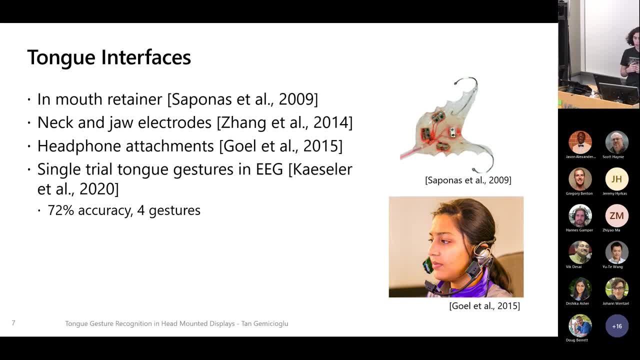 But since then the form factor for tongue interfaces has moved gradually outside the mouth, using electrodes on the neck and jaw and then attachments to headphones that could detect wirelessly the tongue movements. But all of these still required additional sensors. that didn't really. 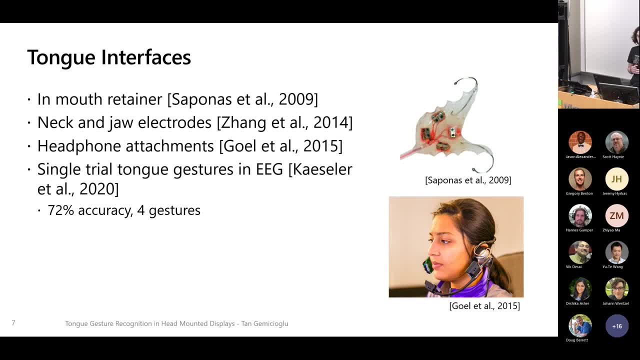 play well with the existing sensors in head-worn displays. One paper that gave us a lot of hope in this area was by Kaysler et al, where they managed to get 70 percent accuracy on four gestures using just a single trial. Leading from that, we were wondering if we can. 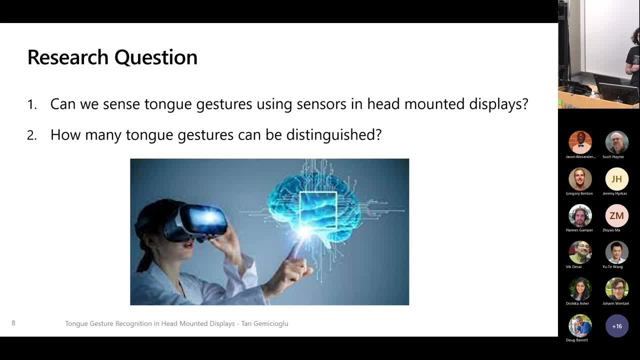 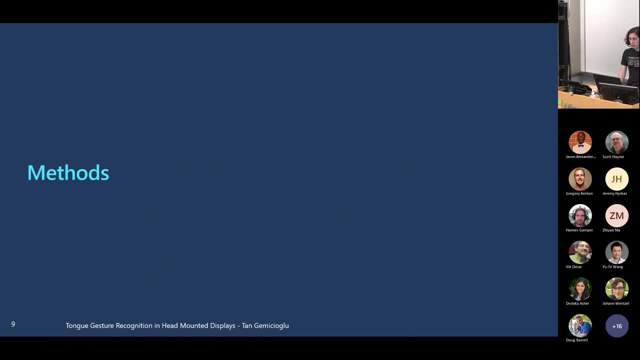 sense tongue gestures using only sensors in head-mounted displays, and we wanted to also see how many tongue gestures can be distinguished using this interface. With that, I'll get started with some of the tools we used to detect tongue gestures. First of all, we're going to talk about the features of tongue gestures. 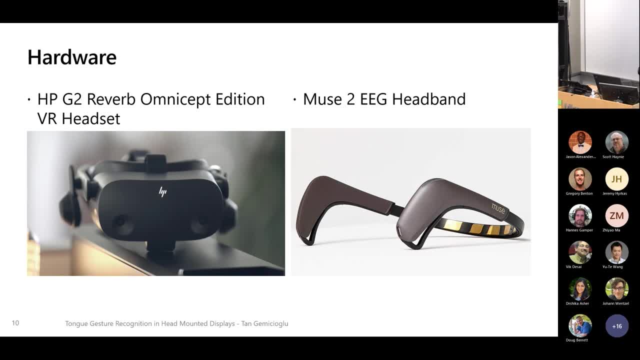 First of all. firstly, we started with the HP Reverb Omnicept Edition VR headset. This is a VR headset that's been kitted with an additional set of sensors, including a heart rate sensor, eye-tracking and various other extra sensors, such as additional IMU. 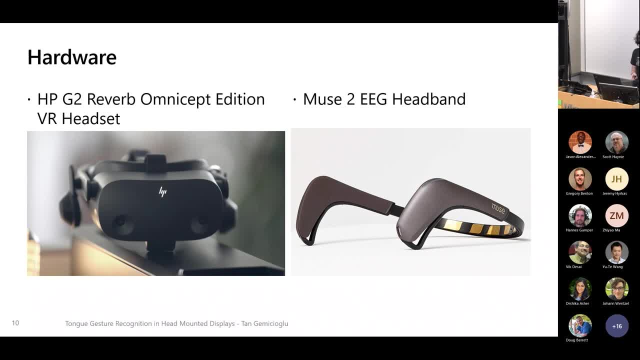 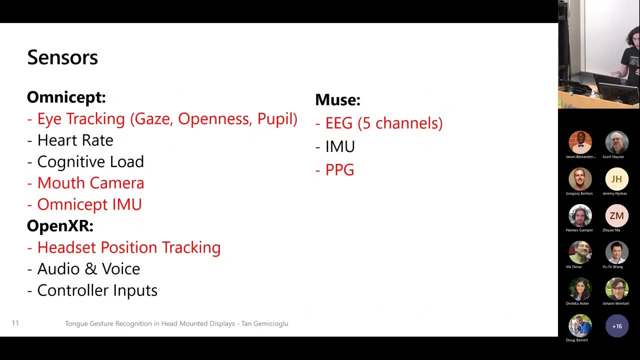 Now we also wanted EEG, based on the past paper we saw. so we used the Muse 2 EEG headband to be able to get the EEG signals. Here's a full list of all of the sensors we were looking at Among these. we weren't able to use all of them. 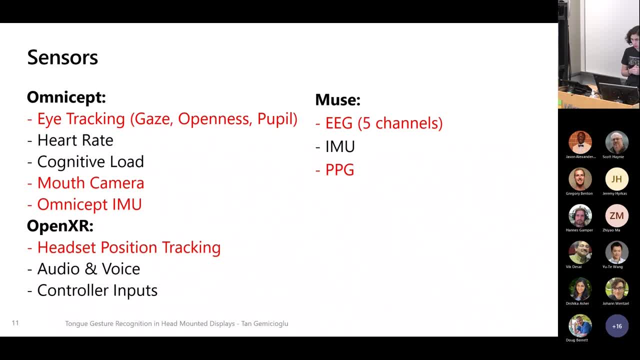 For example, the mouse camera actually was not usable due to the limitations of COVID, where some people chose to wear face masks during the data collection. Also, 50 gigs of data is a lot from the camera. We primarily focused on the IMU, EEG and photoplethysmography. 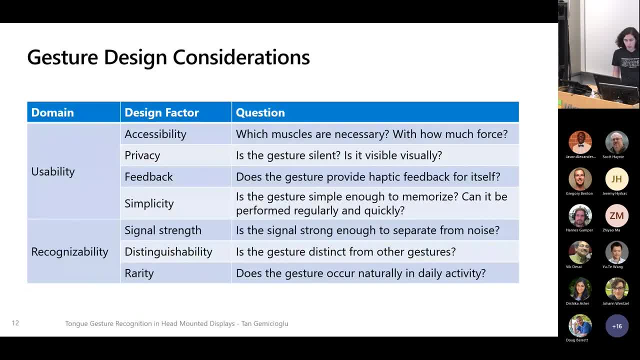 which is used for heart rate detection. In choosing our gestures, we considered a lot of different factors. We generally separated this into usability and recognizability, based on what they were prioritizing. In usability, we looked at accessibility because we wanted to make sure. 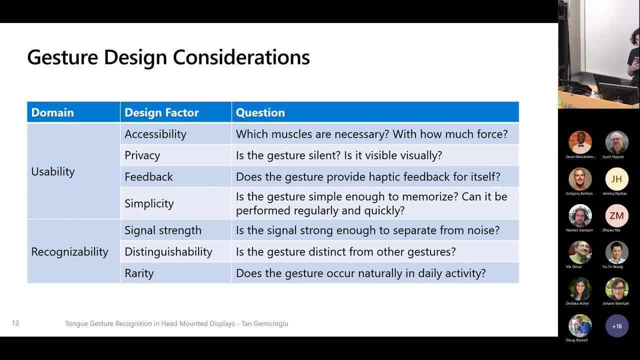 that our gestures were usable by people who did not have a lot of control for their muscles. We wanted these to be private, so that they could be silent and they wouldn't be too visible to someone looking at the user. We also used something specific to tongue gestures. 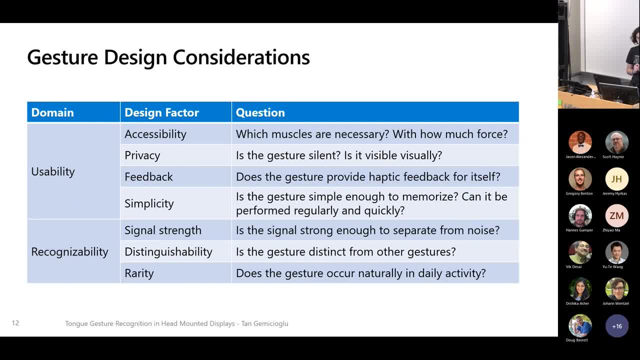 the ability for the gesture to provide haptic feedback for itself by touching the surfaces around the mouth. We also wanted to keep the gesture simple so that it can be performed regularly. We also looked at some different signal processing criteria, such as being able to get a strong signal and. 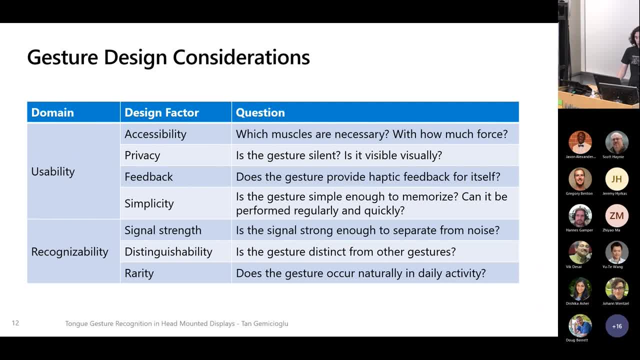 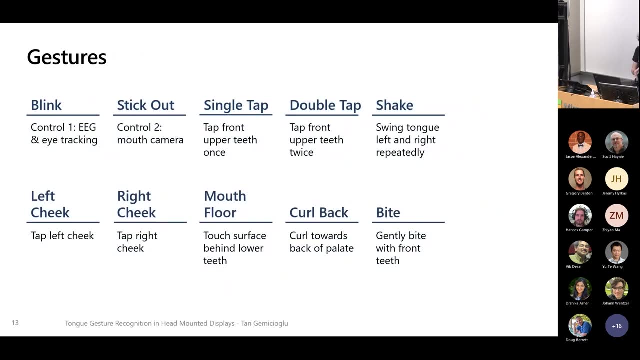 being able to distinguish it from other gestures. Of course, this had to be something that doesn't often occur in daily activity for it to be able to be pendently recognizable. On that, we chose eight gestures and two additional controls to be able to give. 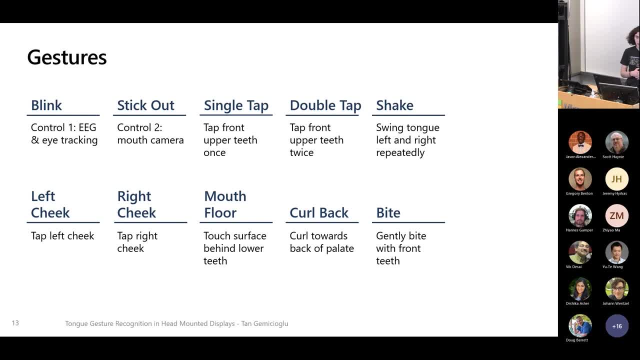 a point of comparison to other researchers on eye tracking and gesture recognition, We used the blink and sticking out the tongue as our two controls. Other than that, we used tap on the upper teeth, shaking the tongue left and right, the cheeks and also some others like the bottom and top back of the mouth. 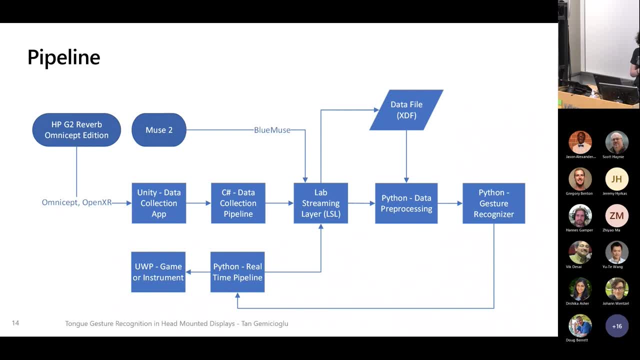 To be able to get our data from our sensors all the way to our processing pipeline, we built a Unity interface which then streamed all of the data over the lab streaming layer and finally put this all in Python, where using scikit-learn. 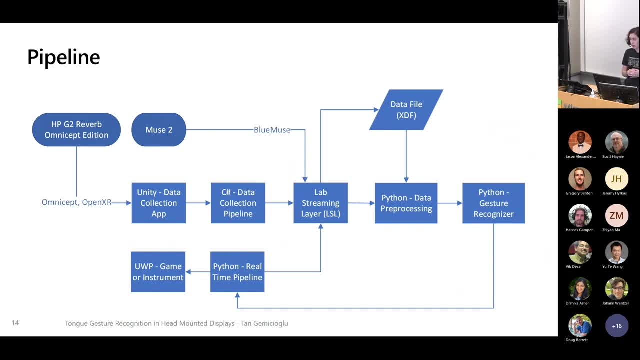 I was able to recognize the different gestures For the real-time pipeline. we also additionally made an interface for the universal web platform and streamed all of the outputs from the real-time pipeline onto the keyboard, which would allow this interface to work with any other application on the desktop as well. 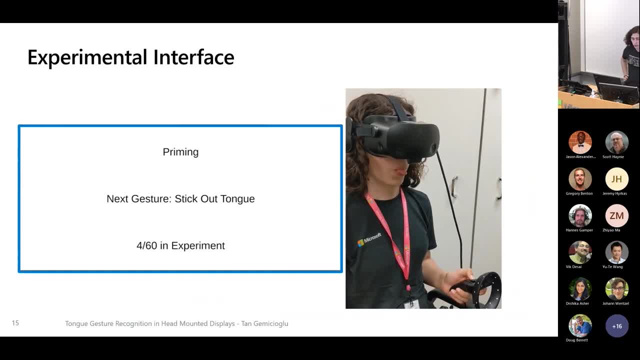 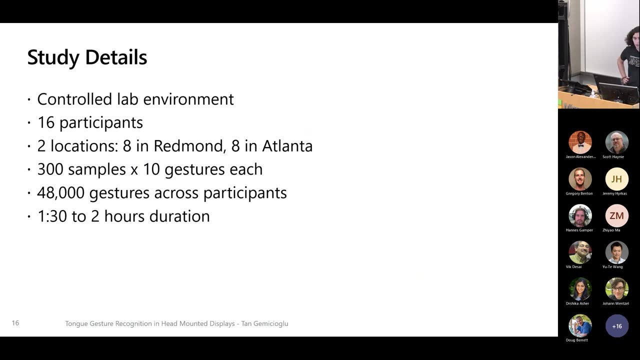 So here's an example of me performing some of the gestures during our experiments. For the study itself, we used a controlled lab environment, so it was not exactly something where the participants would move around and do the gestures, but this still gave us a good 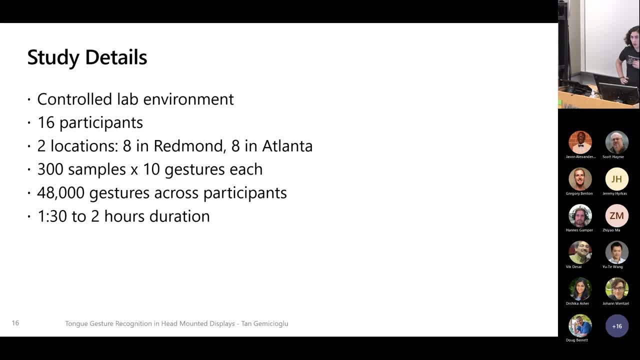 good exploratory foundation on understanding which of our gestures and sensors are more useful, And we had 16 participants in two different locations, equally split between Redmond and Atlanta, And in total each participant did 3,000 gestures, with 300 samples for each of the 10 gestures. 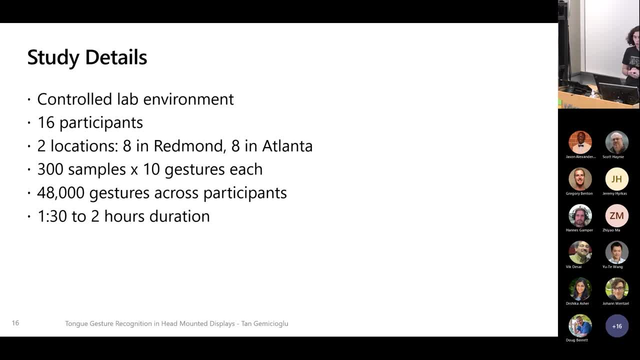 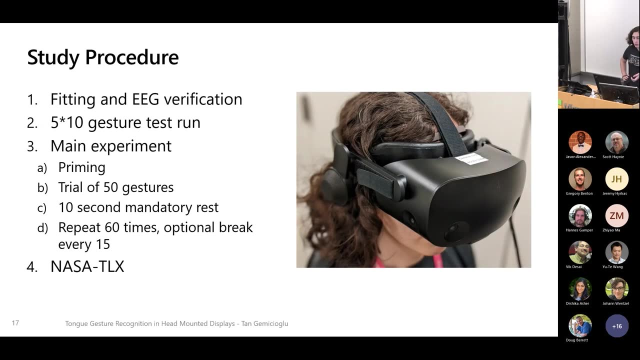 which gave us a really large data set of 48,000 gestures across all of the participants And typically per participant. this lasted about two hours, with some variation of course, And for the procedure we started with fitting both of the headsets. 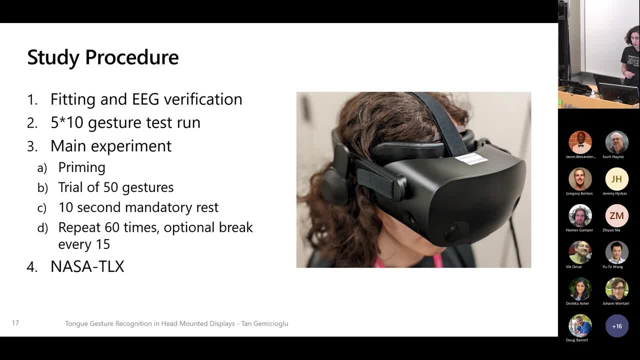 and you can see what the form factor actually ends up being here. And obviously this was not the most comfortable, but since we were just trying to understand which of the gestures were useful at this point, it was useful for us to build a better comprehension and form our data set. 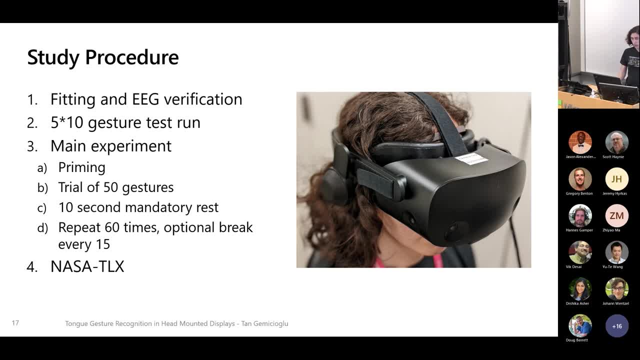 And then we verified that the EEG signals were connected and within normal variance, and then did the test run so that the user was familiarized with the gestures and the pipeline was verified to be working. And after that step we proceeded with the main experiment. 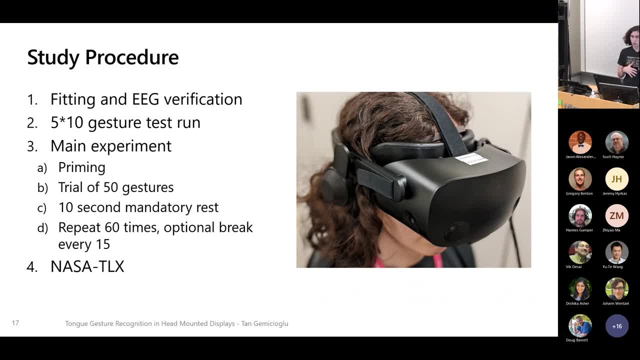 which consisted of a repetition of a priming session where they were shown what gesture they were about to do, a trial of 50 gestures each a 10-second rest session that we kept mandatory so that we could use to detect the rests. 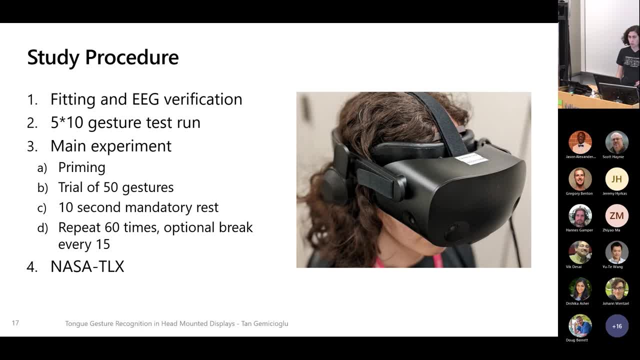 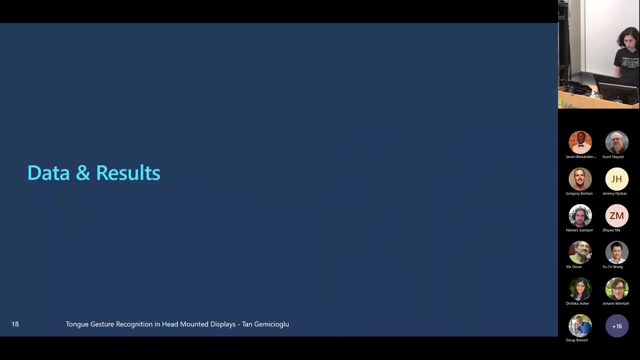 and then they repeat 60 times, with optional breaks in between. And finally, for the participants in Atlanta, we also added the NASA TLX so that we could collect, so that we could collect metrics on the usability of the gestures And for data. let's start with some demographics. 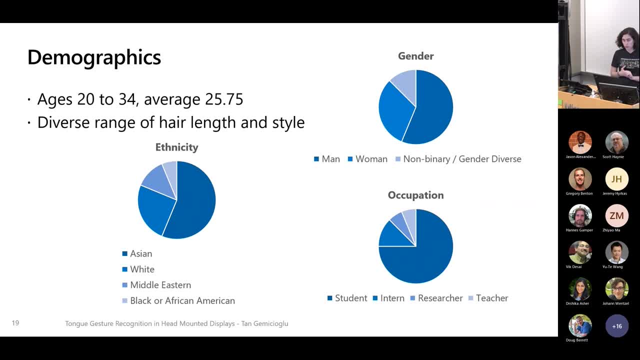 Our participants ranged in age from 20 to 34, with an average about 26.. And as a study that included a lot of EEG signals, it was important to us that we had a diverse range of hair length and style, because many EEG studies fail. 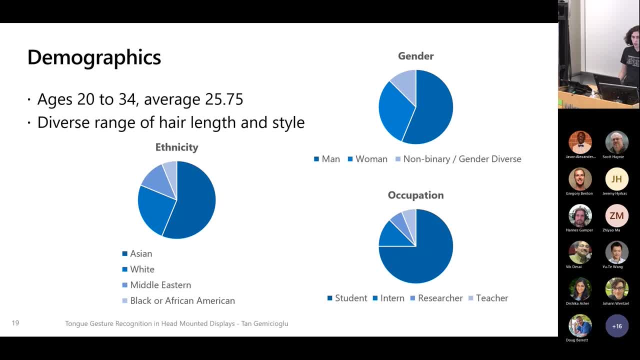 in different hair conditions, But one of the benefits of the MUSE was that the electrodes were actually located in spots where we could still collect EEG data, even when the hair was curly or braided and otherwise. And ethnicity-wise, the population was mainly Asian. 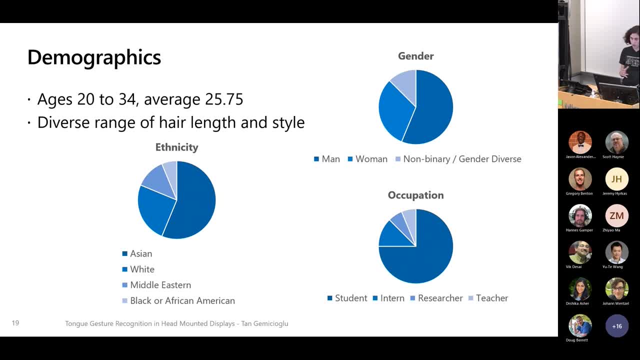 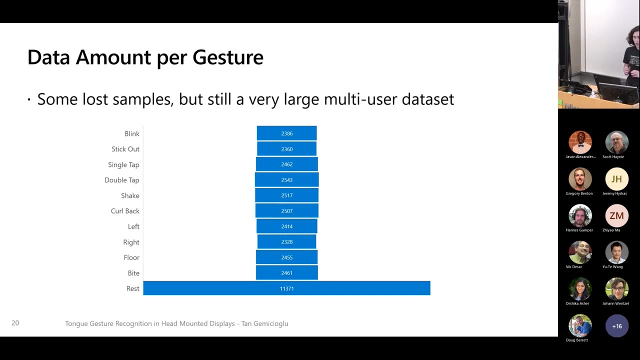 but we had a decent split And gender-wise it was also primarily men, but somewhat more balanced, And most of the participants were students. And per gesture, after applying our exclusion criteria and some of the samples being lost, we still had a really large multi-user data set of 2,400 gestures per. 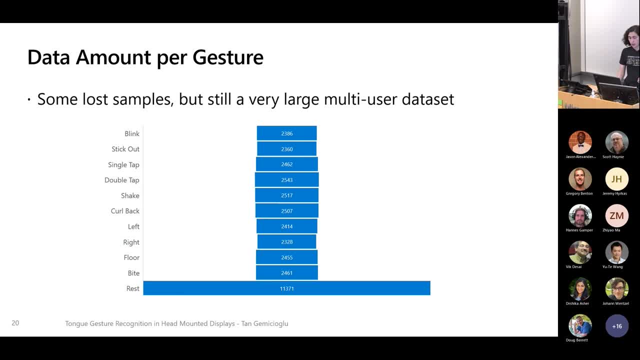 well, sorry, 2,400.. So we had a really large multi-user data set of 2,400 gestures per well- sorry, 2,400 gestures per well, sorry 2,400.. And a really large set of rest conditions. 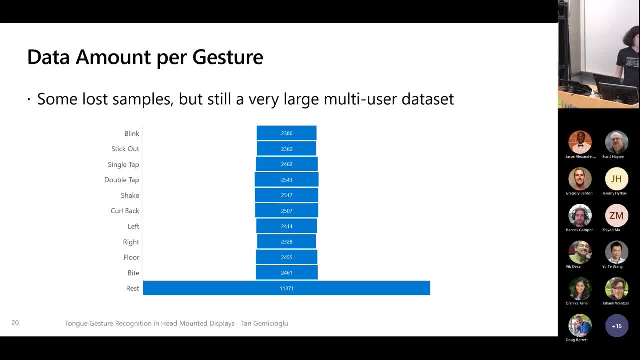 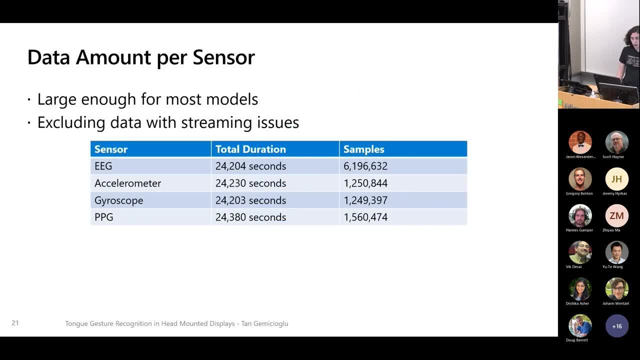 And per sensor. this added up to more than a million samples per sensor, which added up to about 24,000 seconds, which was really useful going forward, because this would be useful even when we used more deep learning methods to answer a lot more of these questions. 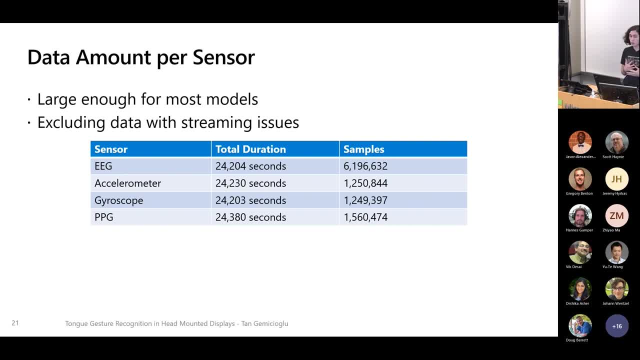 So it was a good study and it was really interesting And you know we learned a lot from everyone, So we wanted to show this to you and give you some tips on how to do this. a couple of things about SLCs: 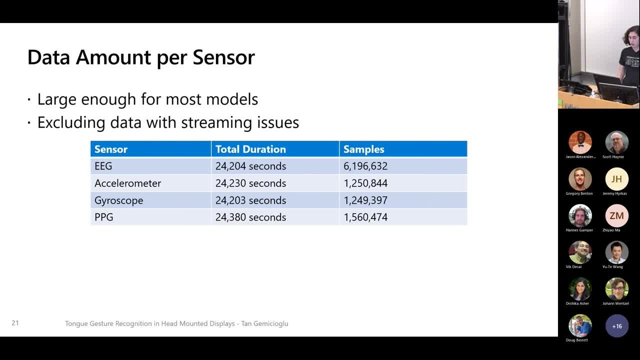 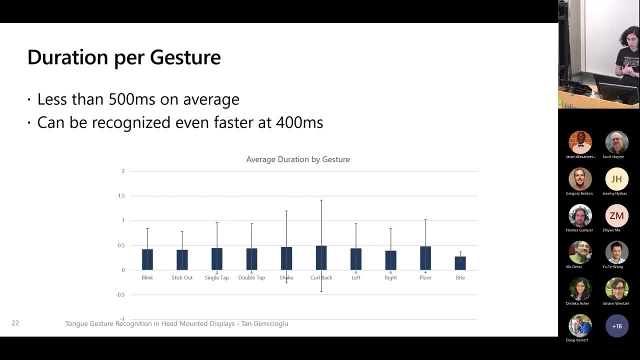 deep learning methods, although for the duration of this presentation we have not reached that step yet, and per gesture we had about less than 500 milliseconds on average, which gave us something comparable and mostly better than gaze and dwell, which gave us a lot of hope. there was some. 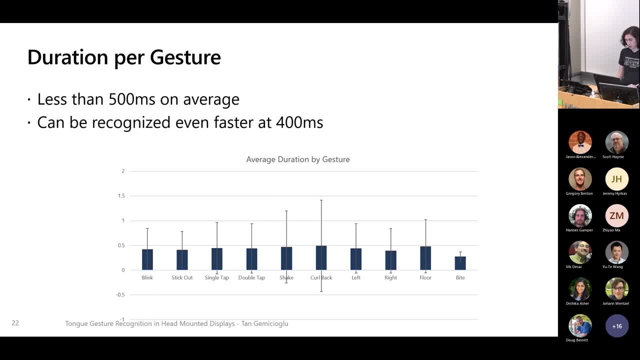 variation in the duration reported by the participants. uh, because, uh, the clicks actually weighed, based on, uh, various users and how tired they were, and in normal applications they would not be doing 3 000 gestures back to back. so we believe that it would actually be possible to. 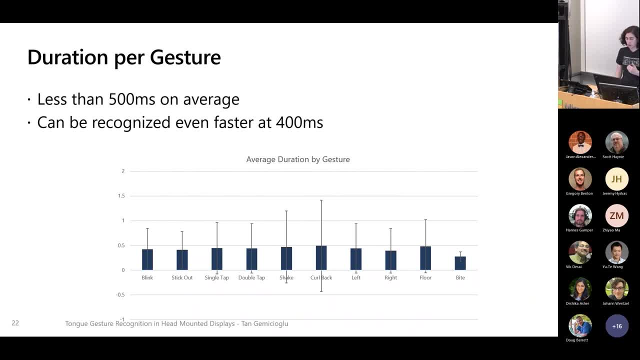 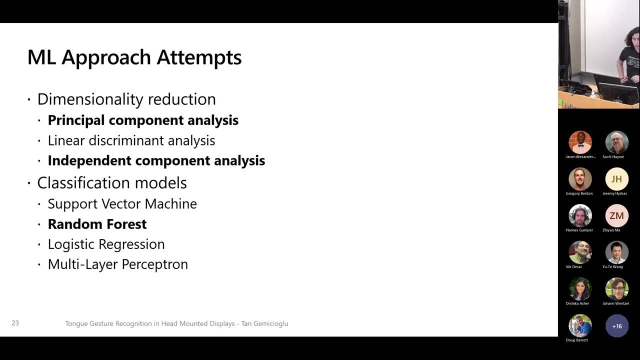 run it faster than this and we actually observed, as we'll uh talk about later uh, that we can recognize uh the gestures faster than 400 milliseconds. and for the machine learning approaches, for this, uh, i primarily looked at different dimensionality reduction methods and classification models. uh, here uh, for dimensionality reduction, uh it's. 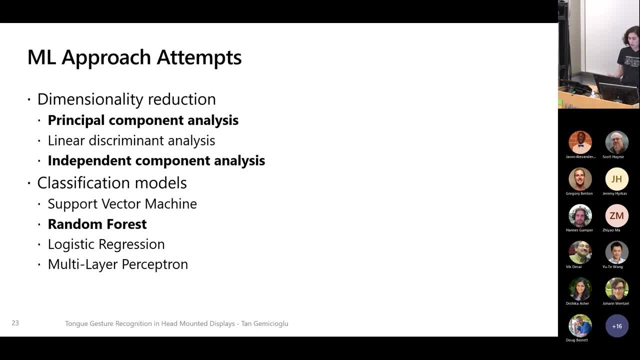 actually diverged by sensor uh for gaussian uh sensors uh like the imu, and uh the photo flatismography uh. um, you can see these uh in the uh, this model uh of like the uh the of the uh uh of the level and by of the number of uh data security measures uh, we are able to uh to look through, but uh. 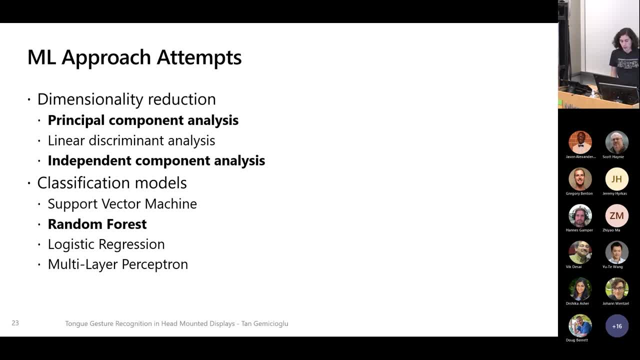 not necessarily, uh, specifically, uh, the ability to uh to uh measure in order to tell the CAD that the cámi is family data about the animal. uh, i don't want to, uh, i don't have the capacity to just look at the data very easily, but, uh, i could go further to the data that the the information. 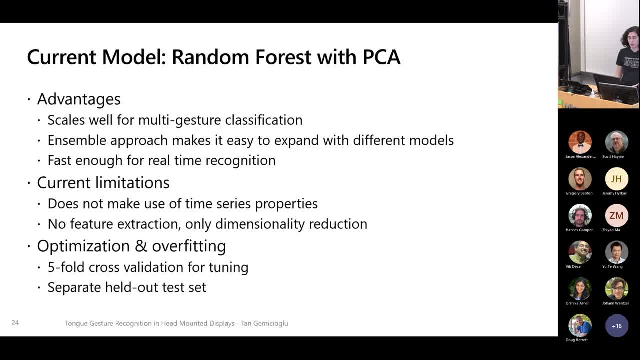 that it's about and do the more detailed analysis of whether it's uh the data within the data set. Generally, we converge towards random forest with PCA approach. Advantages of using a random forest are that this actually scales really well for multi-gestures. 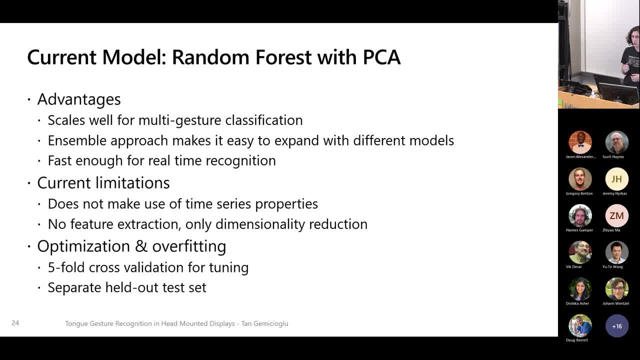 whereas support vector machine is typically better for, for example, binary classification, Because this was ensemble approach where multiple decision trees were fused together. it actually makes it really easy to expand to different models for different sensors if a particular model performs better for them. 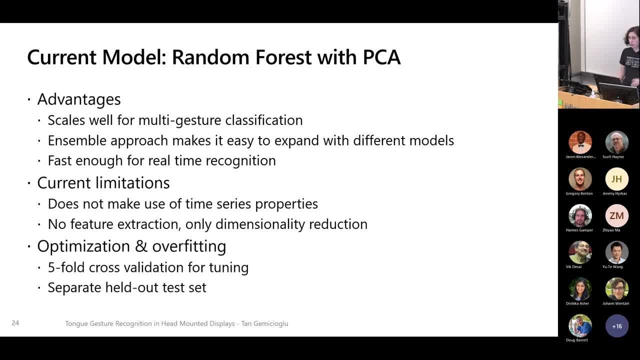 Also, the random forest was fast enough for real-time recognition, which made it really easy to optimize and run. This has some current limitations. currently, of course, and because we just use a random forest, we do not make use of any of the time series properties. 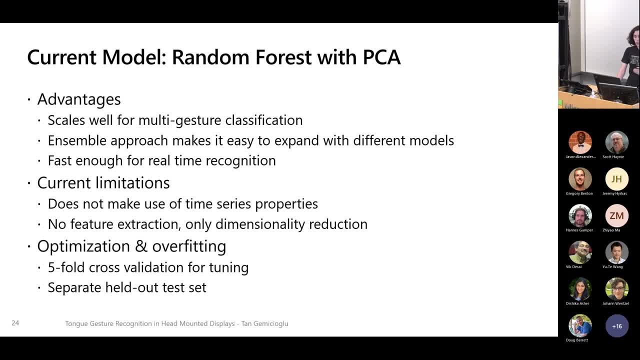 and if we did, the accuracy could be improved even further. The current model did not use any feature extraction aside from the dimensionality reduction techniques mentioned. To prevent overfitting, I used a five-fold cross-validation set for the tuning of the hybrid parameters and had 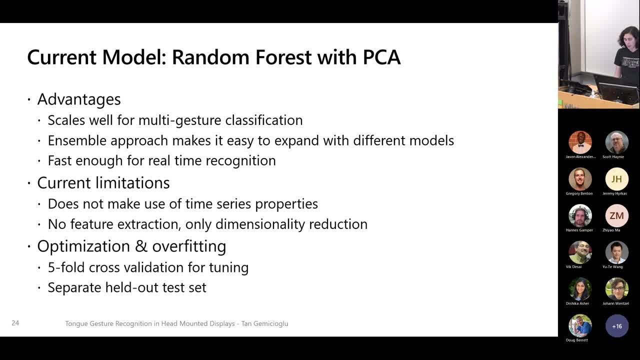 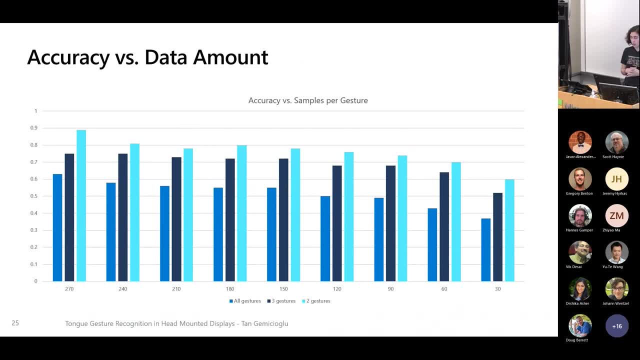 a separate held-out test set for all of the results you will see. So firstly, we looked at accuracy versus how many samples- well, how many runs of each gesture we gave for direct ignition model. Here you can see that it mostly was okay until we got to. 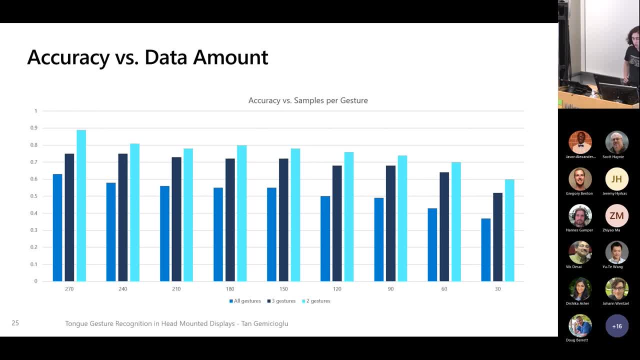 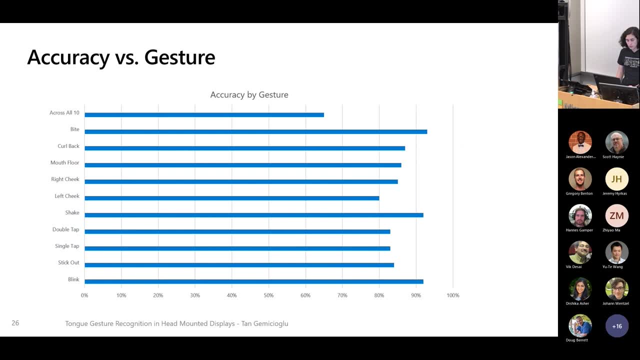 two-thirds and even produced decent results: up until 90 samples per gesture, so a third of our dataset, And per gesture accuracy typically was above 90 percent for some of the more recognizable gestures, such as biting on the tongue or shaking the tongue left and right. 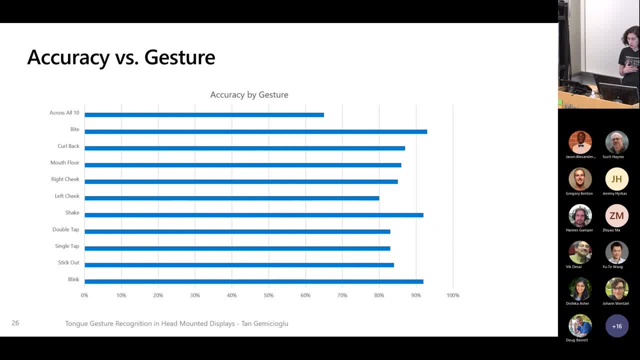 And the blink, as predicted as a control condition, also scored highly. But even for the other gestures we were able to get above an 80 percent accuracy, which got us close to something usable. And if we tried to classify across all 10 of them, 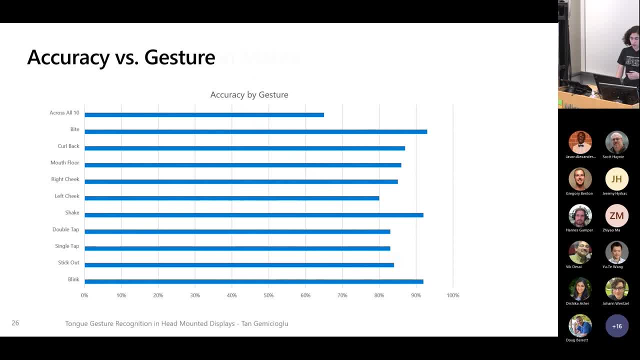 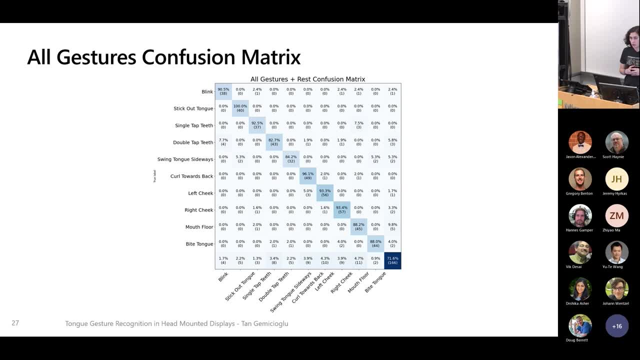 we got about 60 percent And you can see a confusion matrix for that here. actually, Something that gives us hope for the classification across all the gestures was that most of the problems in the confusion matrix were shown in comparing the gesture versus the rest condition. 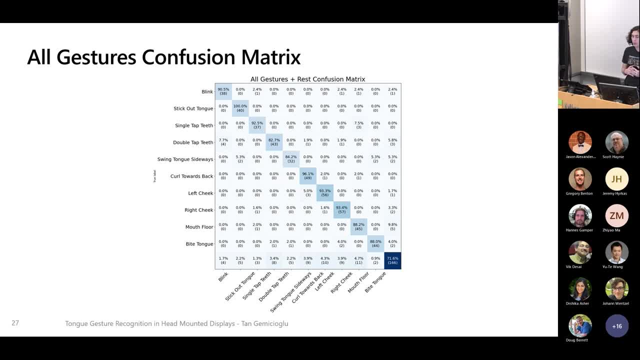 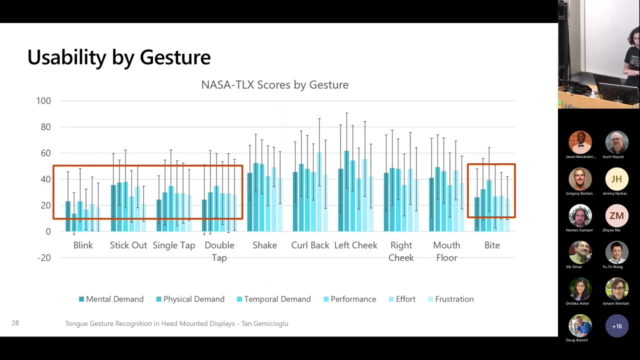 which means that if we improved to have a better rest condition that covered a more diverse range of default interactions, then we would actually be able to improve our accuracy pretty easily. And, based on the NASA TLX, we also looked at the usability per gesture. 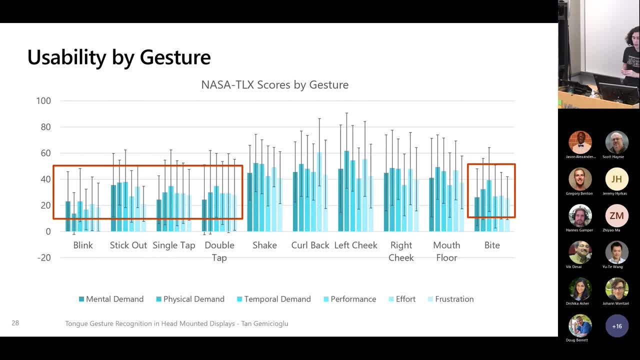 and we found that the single-tap, double-tap and bite were comparable to the blink and stick out control conditions. So we decided that these would be our most usable gestures, And even for the other gestures, despite the high variance. 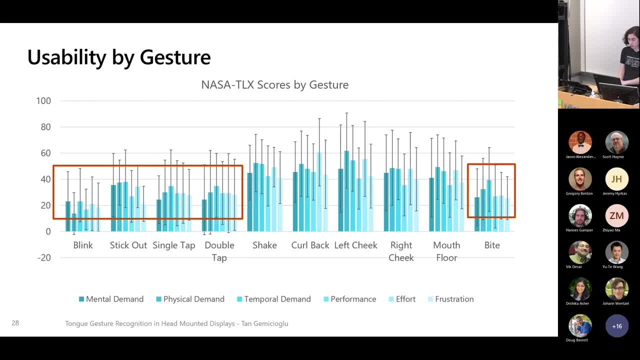 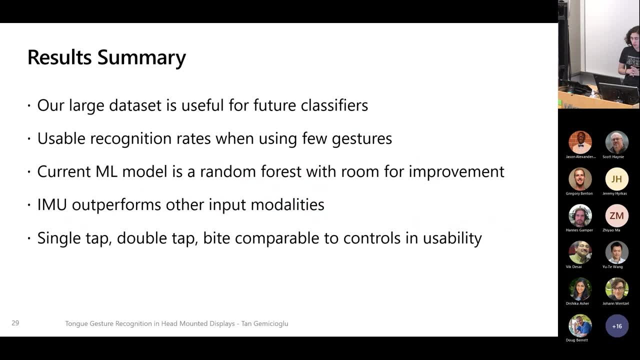 they were still within the range of the other gestures. And to summarize all of these results, we made a large dataset that would be useful for future classifiers. in tongue, gesture recognition And usable recognition rates were possible even with the current models using few gestures. 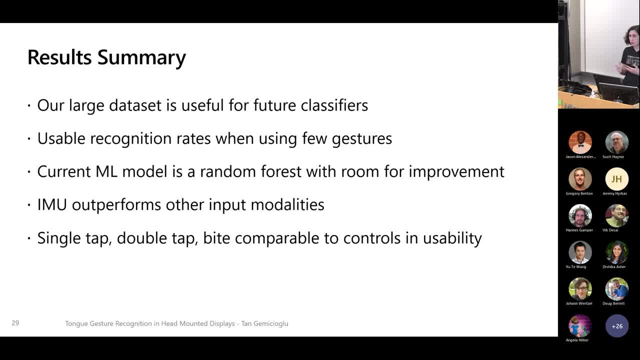 And obviously the current model has a lot of room for improvement and we primarily focused on the dataset and the sensors for the duration of my internship And the IMU outperformed the other input modalities and this was especially interesting to us due to how 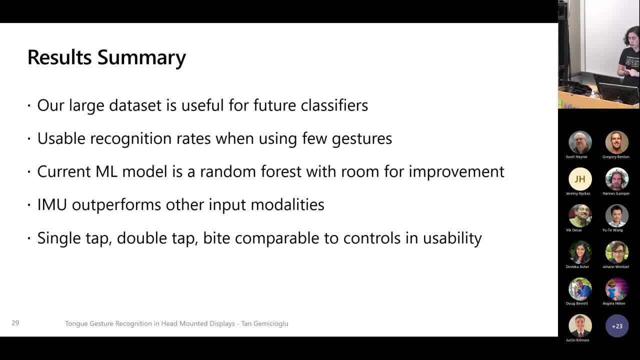 how easy we can put an IMU on different devices, And we also found that single-tap, double-tap and bite were very usable and comparable to blinking, which was why we proceeded with that for our real-time implementation And for the real-time implementation. 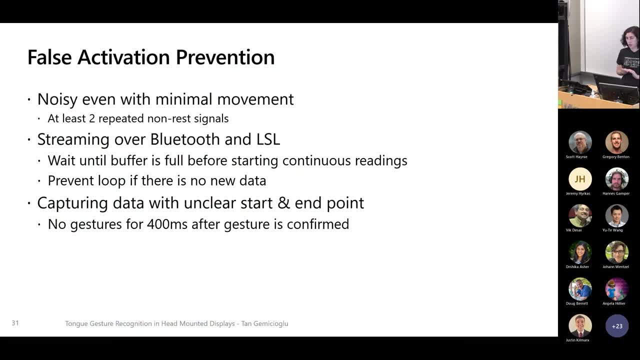 we had to implement some additional measures to prevent false activations due to the noise and movements or the environment, And for this I made it so that it requires at least two repeated non-rest signals before it accepts a gesture being performed And due to the streaming being over Bluetooth. 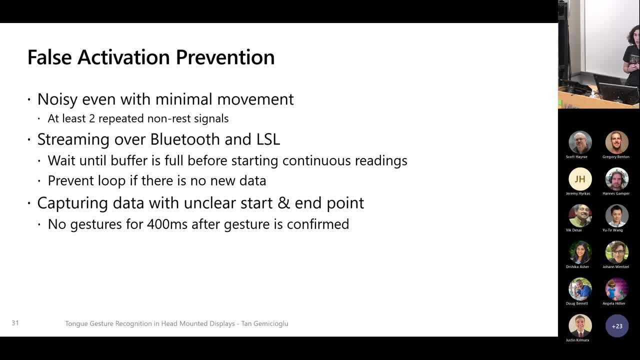 we had to make sure that the buffers were filled and there was enough samples for prediction to be able to be obtained. So I waited for the buffer to be full before continuously reading from the buffer, And if there was no new data, I avoided running it again, so that the loop didn't cycle too quickly. 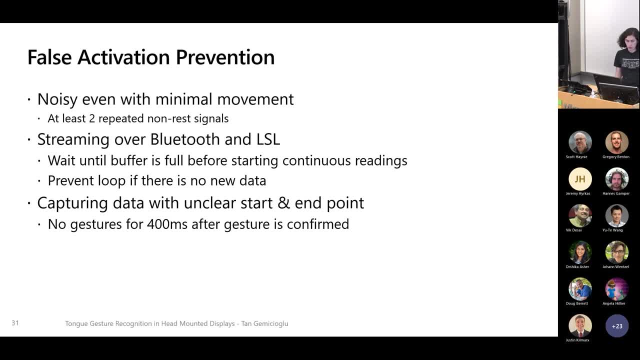 And there was also an issue with how we were capturing the gestures, because we were finding it between longer durations of rest signals And we- I- made it so that there was no gestures for 400 milliseconds after a gesture was confirmed to be recognized, to prevent repeats of the same gesture being triggered. 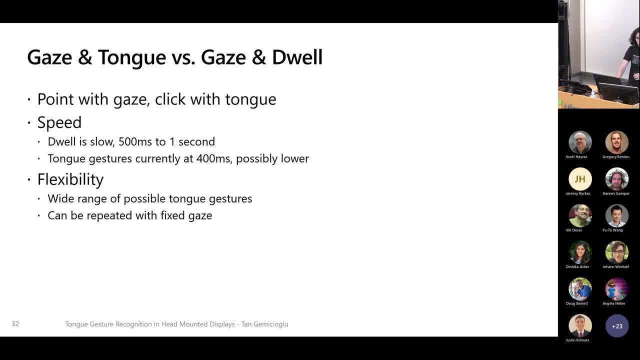 And a lot of our focus in this area was on seeing how gaze and tongue compared to gaze and dwell, And you can think of this interface as using the gaze as your mouse movements and the tongue as your click, Similar to how you can left-click and right-click. 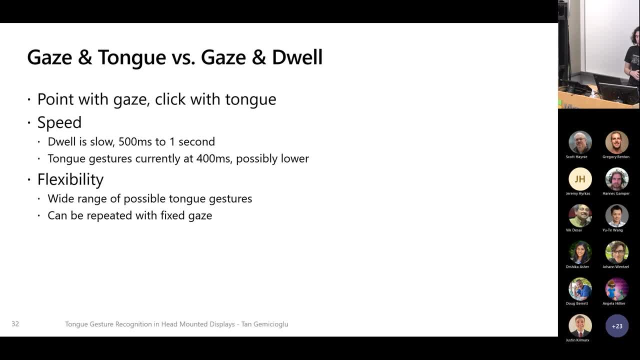 the tongue actually provides more usability than Dwell in flexible settings where you might need to perform different actions on the same location. Also, it was faster than Dwell, which typically ranges in 500 milliseconds to one second, whereas we made it 400 milliseconds and could. 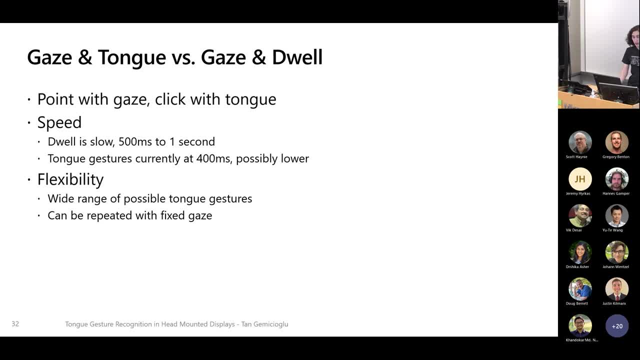 even potentially reduce it to lower than that. Also, the tongue gestures could be done at the same spot with a fixed gaze, whereas Dwell would simply interpret it as a continued Dwell if you fixated on the same spot. So now we can take. 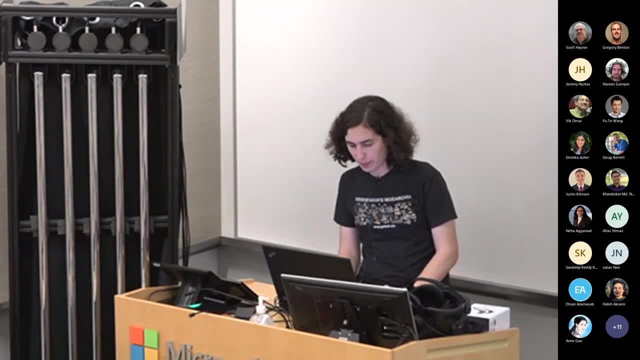 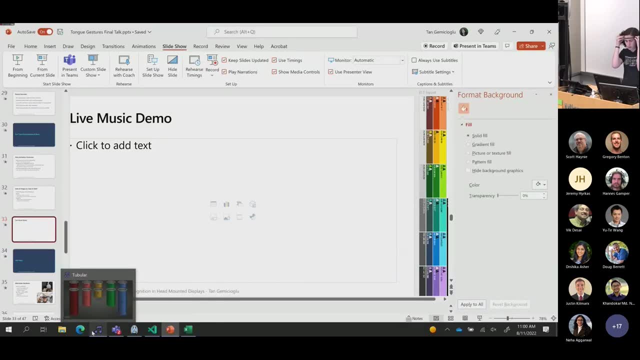 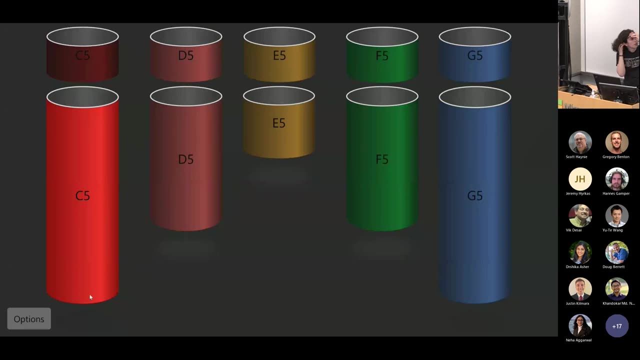 a short break from the presentation for a live demo, and for this we will be using the instrument you can see here on the side. This is played by an app developed by the Enable Lab using gaze tracking, and we provide switch inputs to our tongue gesture. 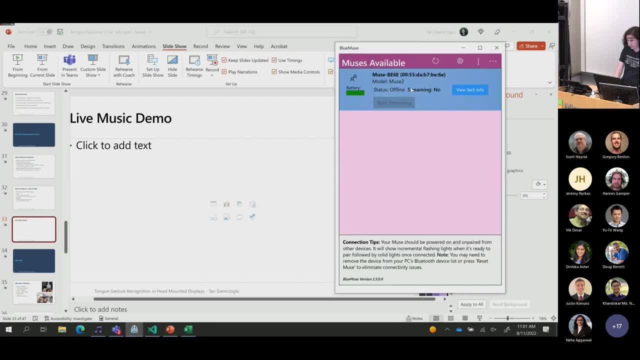 The structure of the punishing system actually makes it easier for us to play with our tongue. What we really do while playing with our tongue is to fit the tongue into the recognition system of our tongue. On the right side of the screen you can see that we have our tongue now on a. 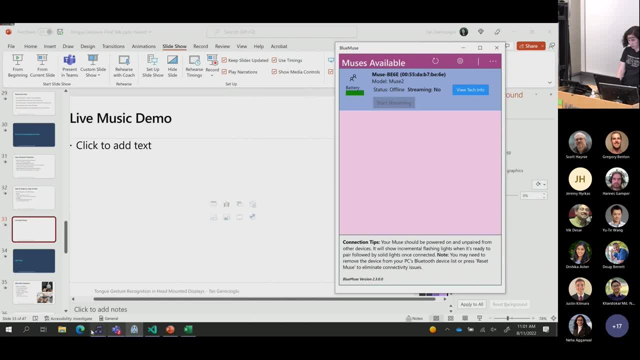 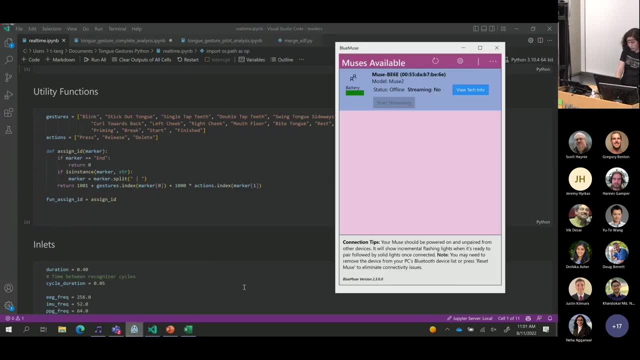 scale. However, we can also use our tongue, which is the projective binary recognition system. We also want tosk at the tongue that is created to play with our tongue, or even put it on a scale that works with our tongue To try to play with our tongue. 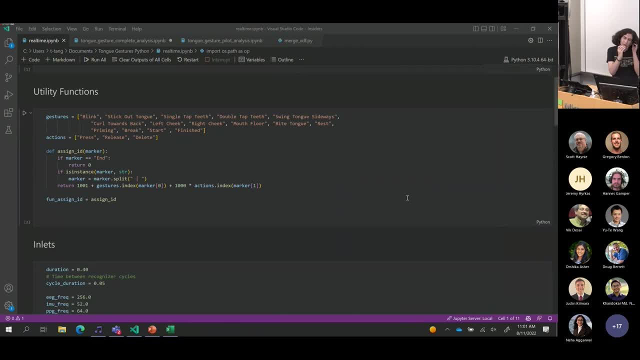 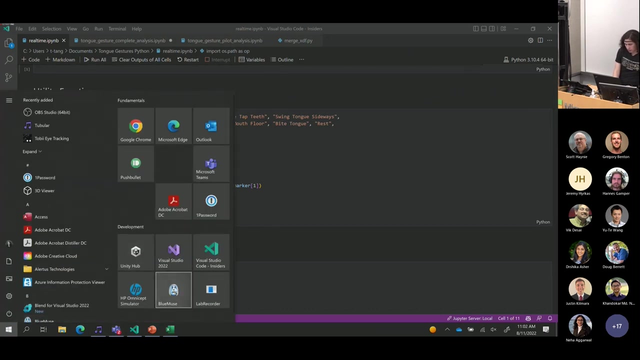 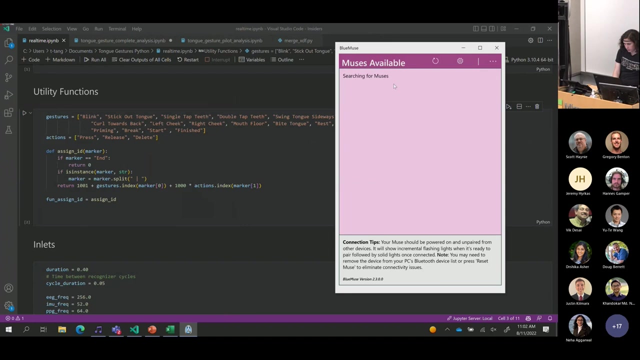 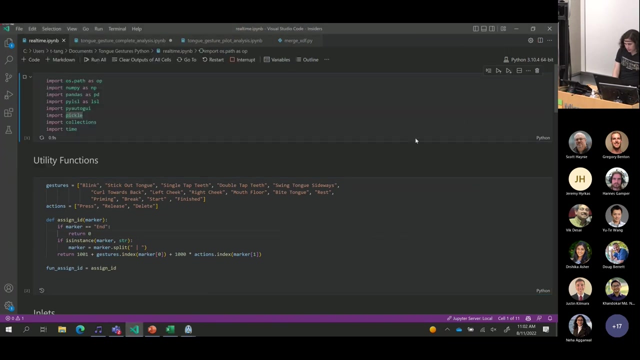 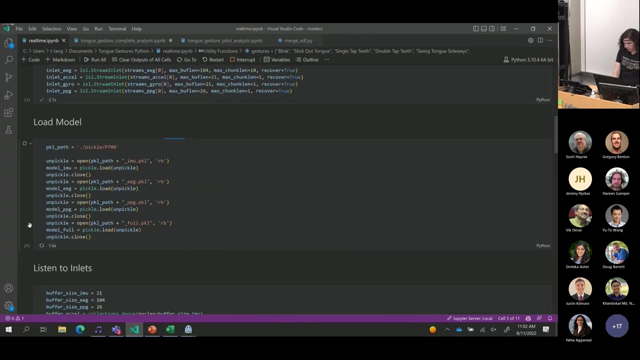 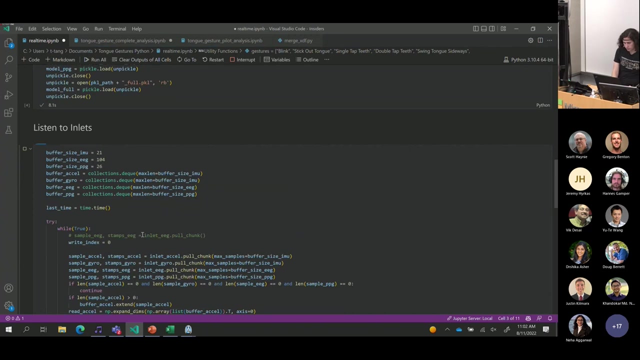 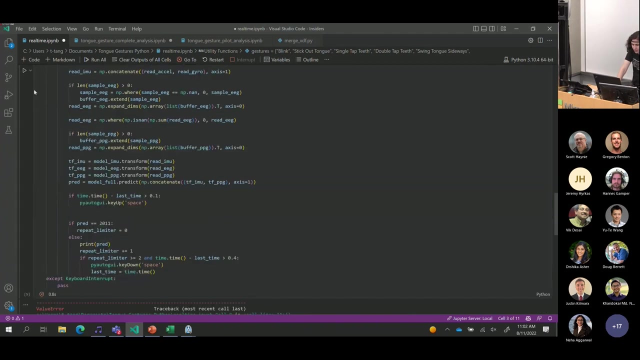 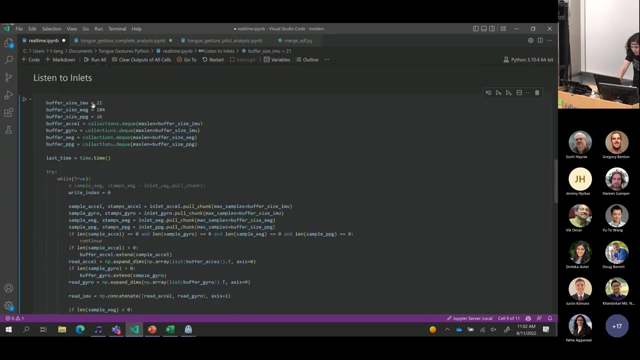 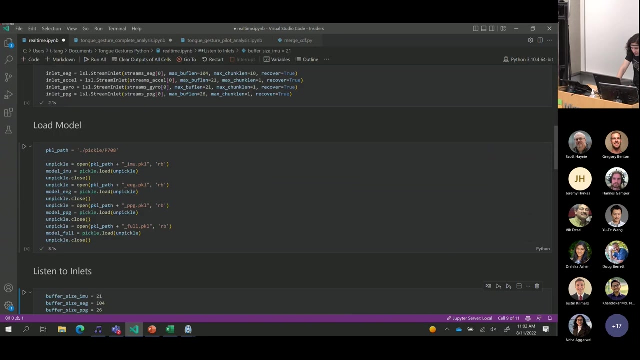 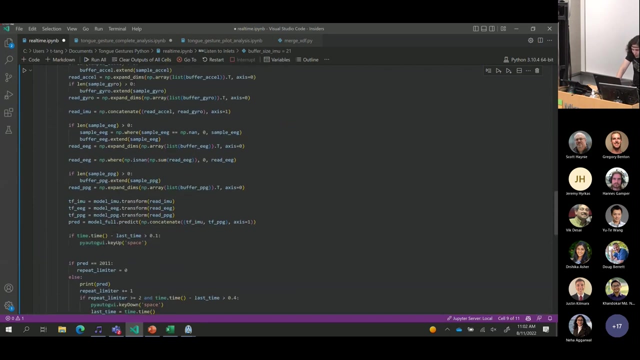 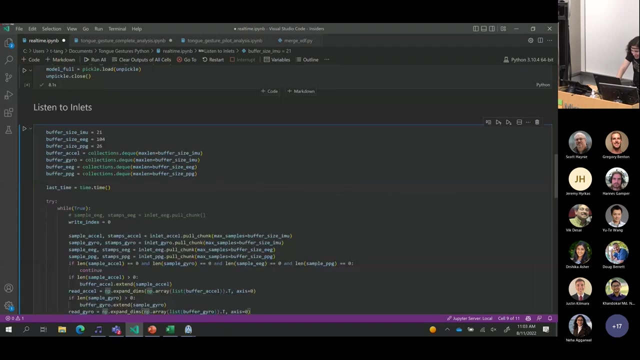 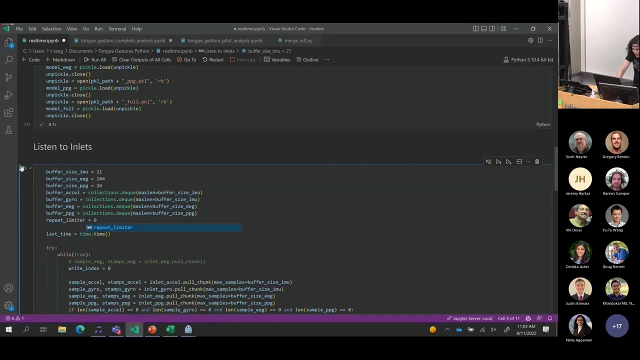 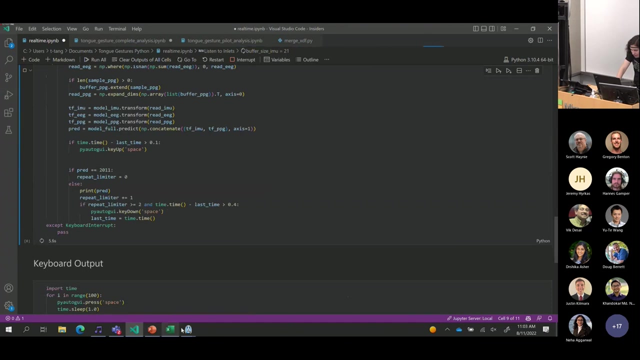 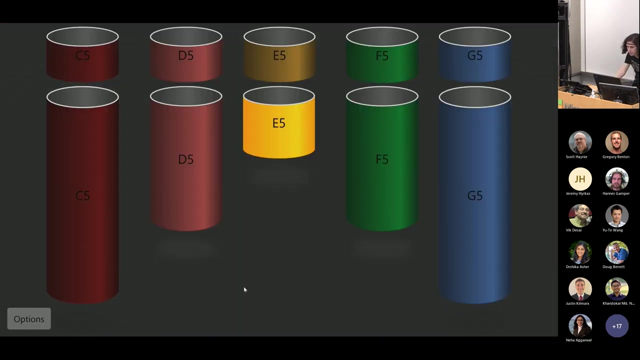 we'll use a voucher. This might take a moment to set up, but I promise it's worth it. Thank you. Some quick technical difficulties due to the course of demos. All right, and now we are streaming. What do the labels mean? 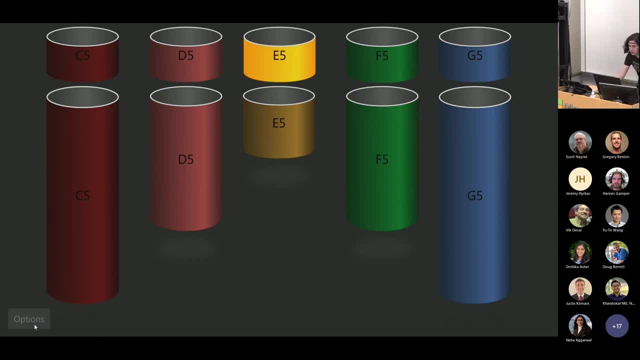 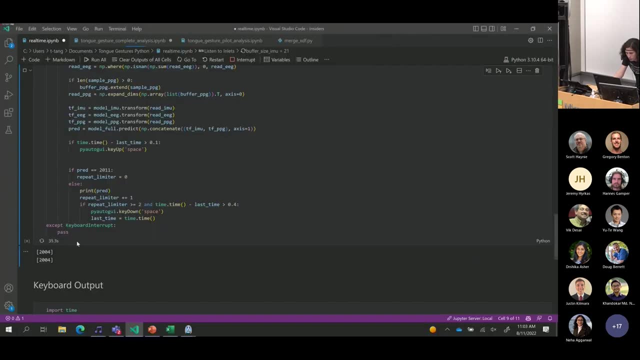 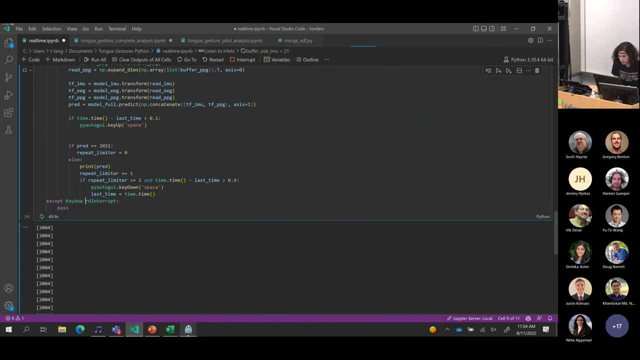 Um, those are the musical notes. So C5, D5, E5, they line up to these. Let me first make a quick test on here because, as I said, it diverges a lot by environmental noise. Okay, Okay. 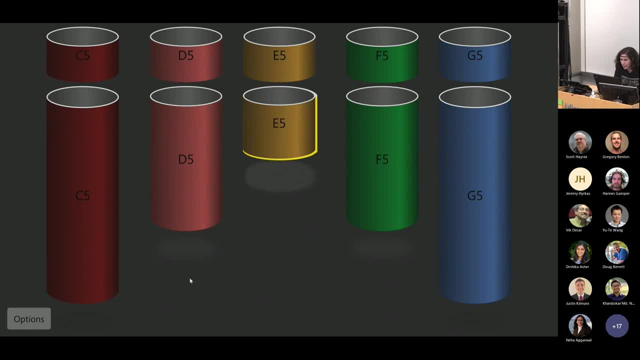 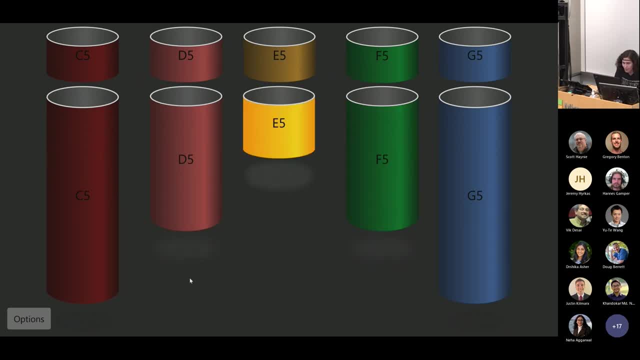 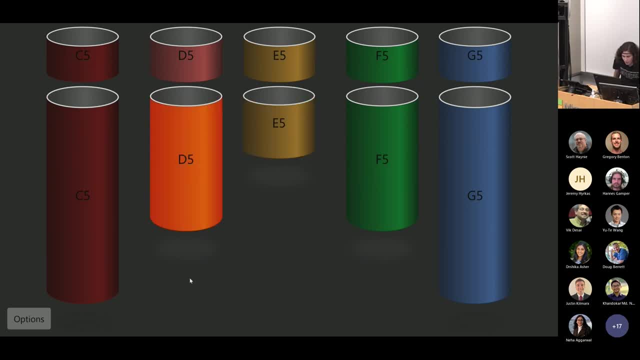 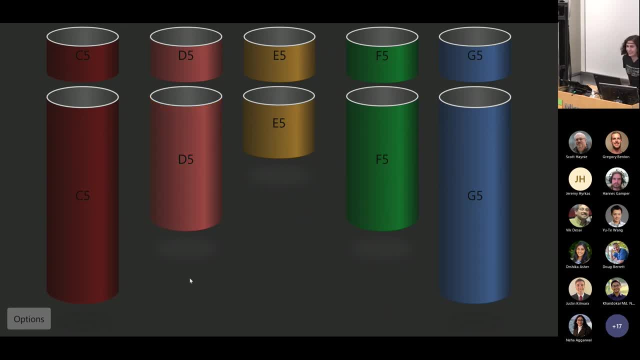 actually alters the signal by quite a lot. Is the eye tracker calibrated? The eye tracker is somewhat calibrated, but not for my position. Can you explain a bit more about how is it controlled? the control- so you look at the eye-tracking looks. 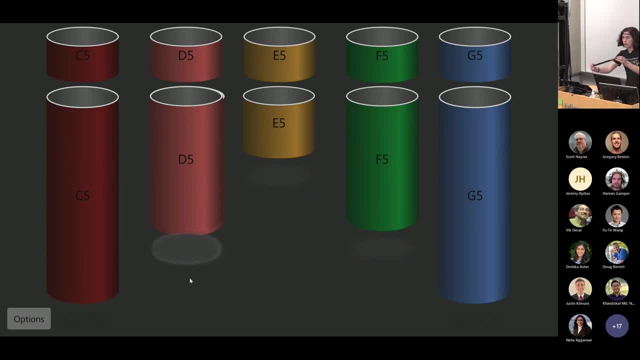 Yes, to show it to everyone, we use Tobii eye-tracker on the desktop currently, and this is combined with the EEG headband I mentioned, which senses the tongue gestures, streams it to the desktop and then streamed over Python onto the keyboard. 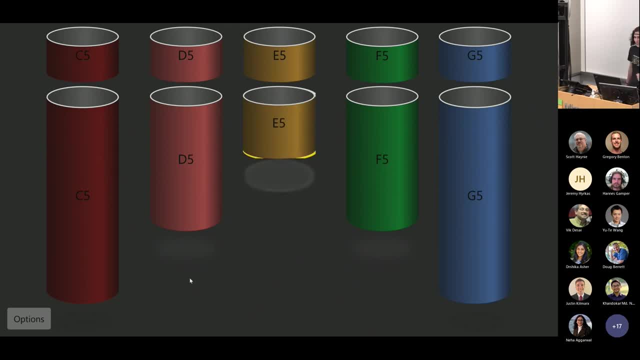 which then triggers responses within this app. Remarkably few false positives. What's the difference between the upper and lower? The upper and lower were actually designed for Gaze plus Dwell, and we don't even need those when we are using Gaze plus Tongue, because I can just look at. 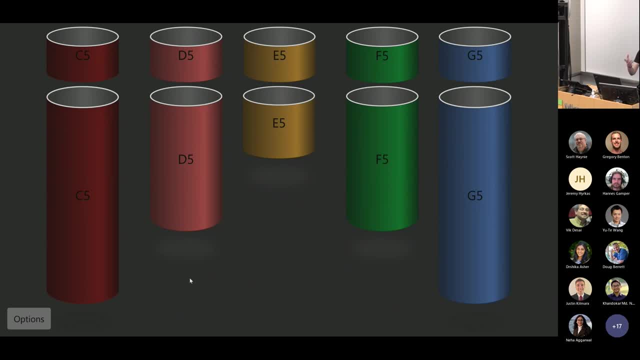 the same one and trigger it multiple times. But when it was Dwell, they had to look between the two so that they could trigger it twice in a row. What was Dwell? Dwell is a method of sensing using eye-tracking. Yes, Nullify a little. 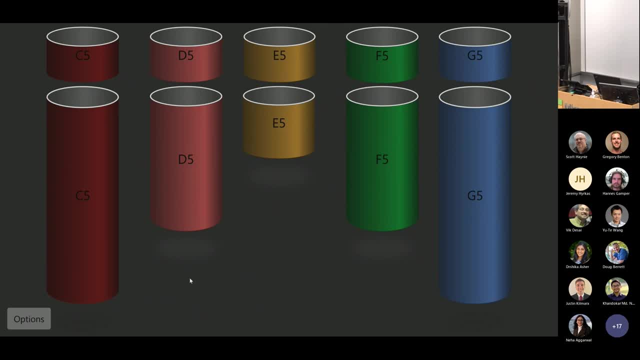 Yeah, Dwell uses your fixation on a single spot to trigger a signal, whereas when we just use gaze tracking, we use it for the location but not the triggers. So you're trying to trigger each one of those in your demo. Yes, Currently this is O2Joy. 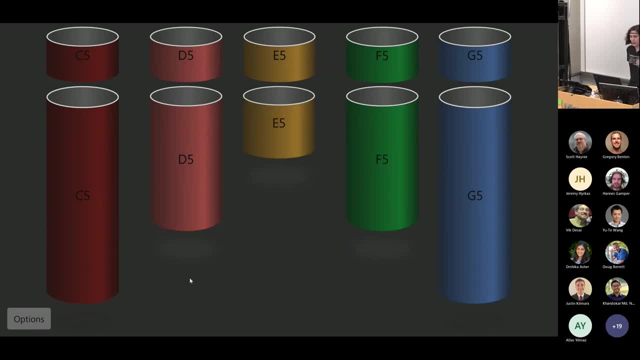 and you got the first few notes, but then it diverged due to me shifting my head. We're trying to do O2Joy. You're always using the same tone, just the same thing. Admittedly, it's squatting down and didn't calibrate. 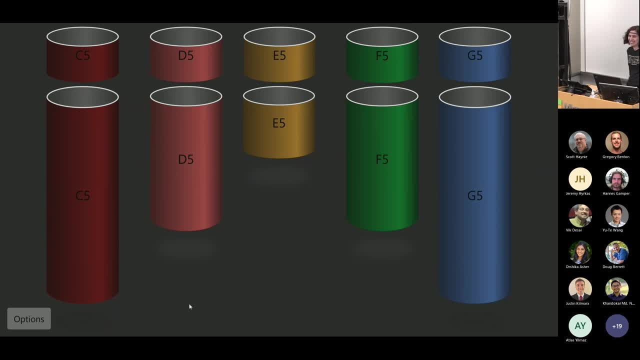 It's very impressive, Nice work. First, tongue virtuoso. But yeah, Speaking of tongue virtuoso, speaking from experience after trying this out, it does require some adaptation to use a gaze and tongue gestures at the same time, because you're trying to essentially 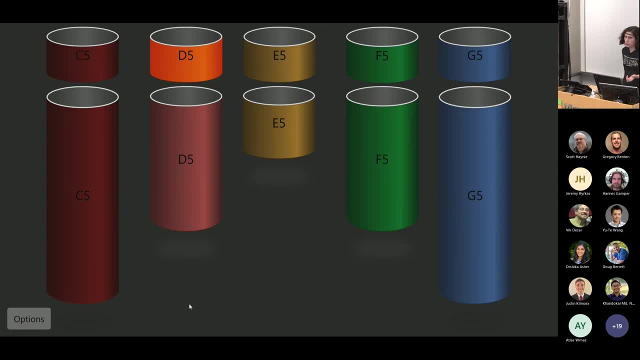 operate two things at the same moment, but it does provide a lot more control compared to Dwell. You are recognizing only one tongue gesture here. Yes, Yes, Here, this is detecting double-tap Operate. Yeah, Yeah, I can do another attempt. 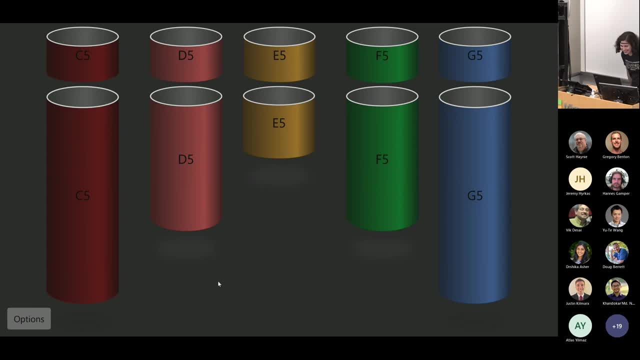 or if we have any questions from the audience. Try it again, Try calibrating, Try it again. I wanted to give you a chance to do it with you. Thank you, I'll take Anas's question. Okay, Yes, Maybe let's do a calibration. 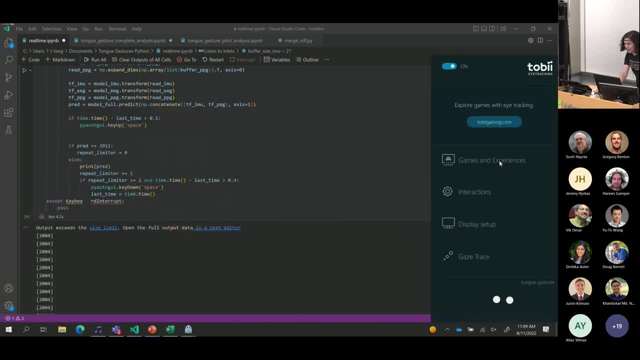 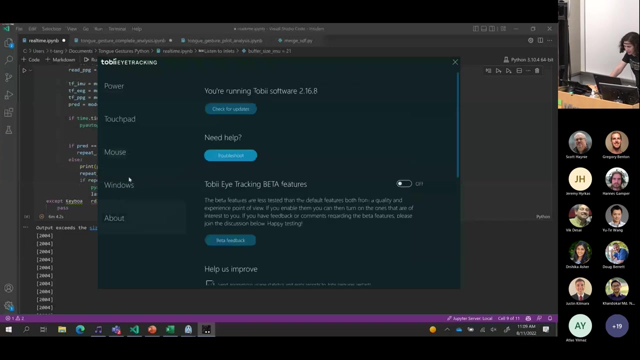 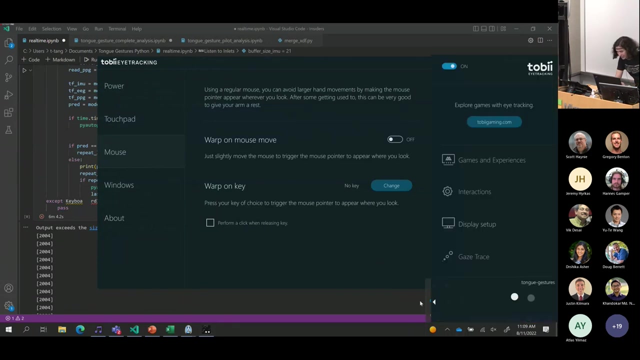 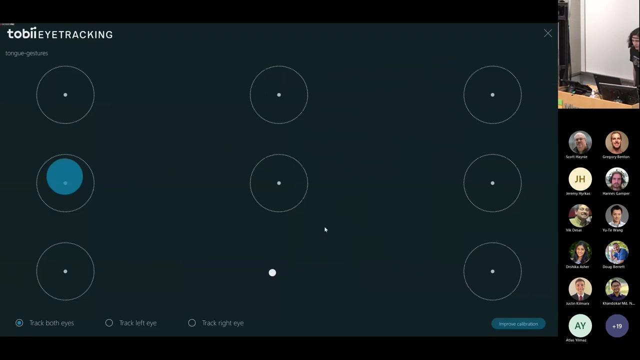 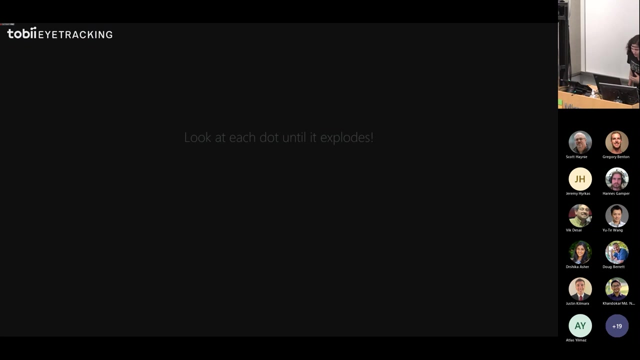 Also, it looks like you added some space in your Q2 working room. Yes, That always happens. Where was it again? Yes, Thank you. Okay, All right, Thank you, Yes. Yeah, This position is not ideal for eye-tracking demos, obviously. 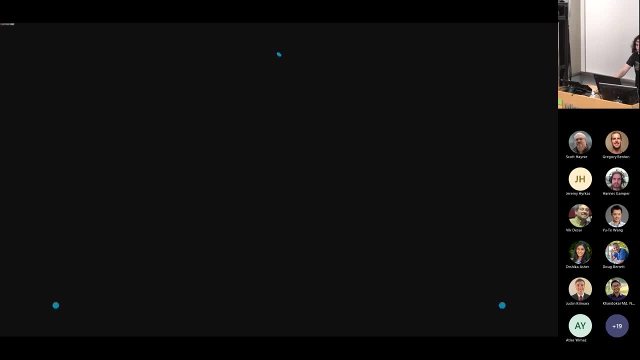 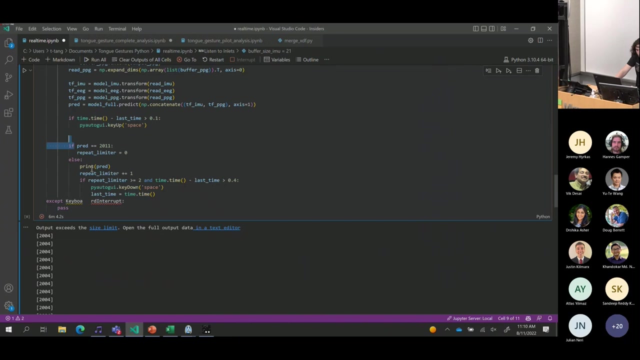 But I am glad you at least got to see half the piece regardless. So now you're calibrating the eye-track here. Yes, All right, I will need to restart this And wait for it to stabilize for a moment. 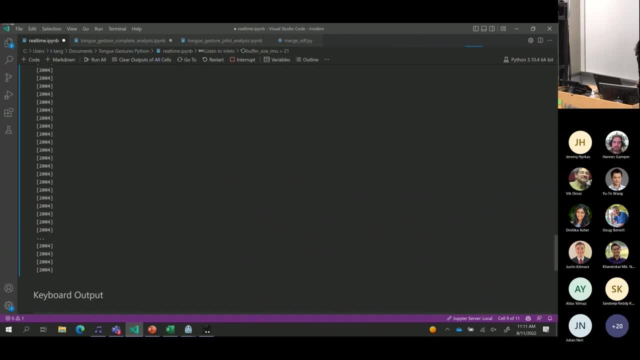 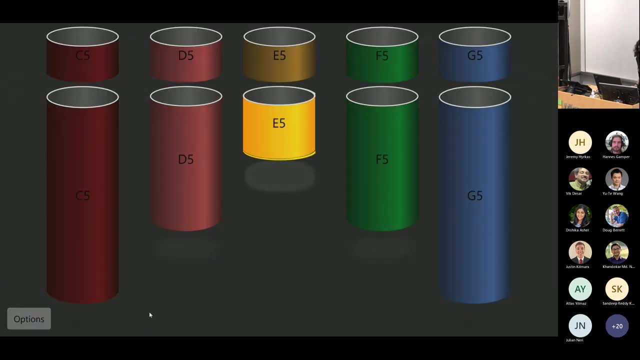 Okay, Thank you. Okay, it's moved off a little. We can get past the piece. keeping it stable for the entire piece might be a bit much. 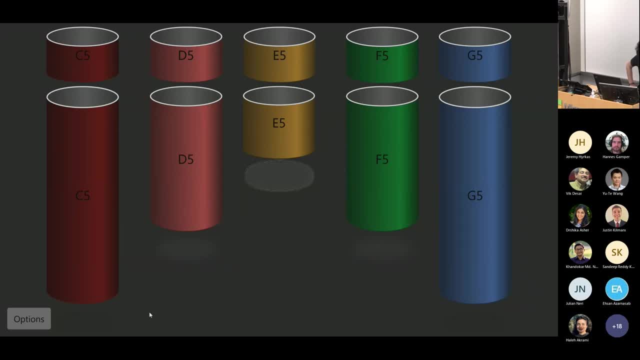 That's the eye tracking, though that's hosing you, not your tongue gesture recognizer. You're probably getting interference from these lights because that's an external tracker, where if you had an HMV with an eye tracker inside of it, you would not have that. 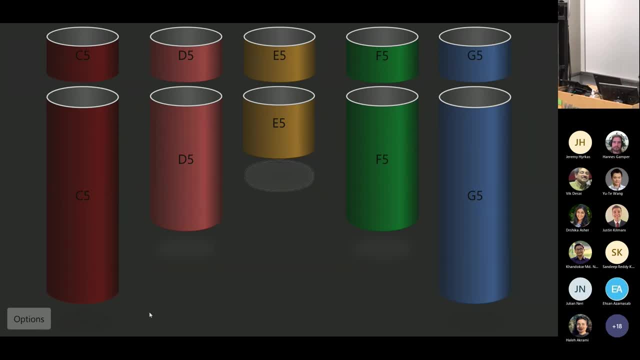 And this is why we were really hopeful when we saw a VR headset with an eye tracker within it. But any questions from the audience online. What's really great about this is that it's super fast and it enables you even to play a piece of music. 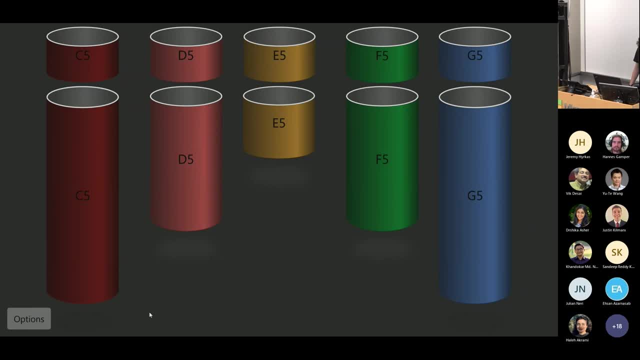 It's a fast tracking technique. Yeah Well, we didn't actually have very much time for data analysis, but we expect that with some more time, we could probably get even better accuracy than what we have here. Yes, Okay, Goodbye eye tracker. 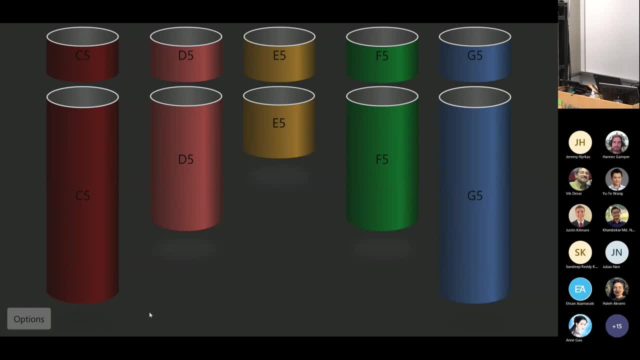 This is why I also emphasized the the elements with the data set, because we could easily improve on the models here than what I did within a couple of weeks. So I want a question on the cross-validations Also. this is you just trained? 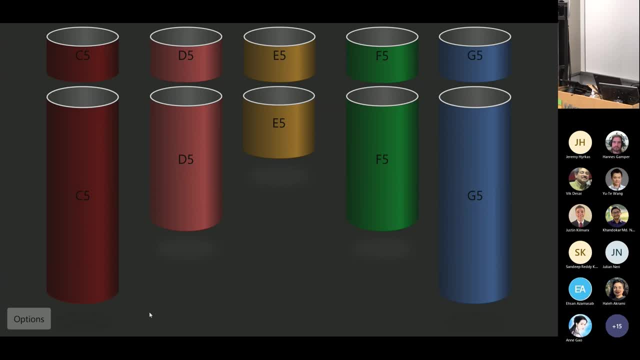 per participant, right? Yes, this is per participant. Check on cross-participant. So for cross-participant, we haven't. we haven't experimented with that as much as of yet. Eventually, I think a user independent model would be really useful. 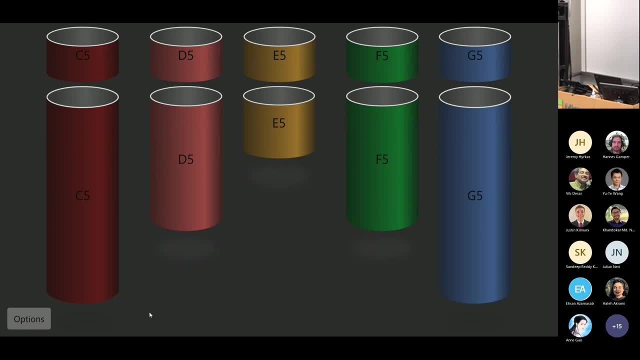 but user independent models with EEG are especially hard typically, So that would require a bit of experimentation to see if it works. Oh, I had a question about the usability. You were talking about the usability of the different, the different types of gestures. 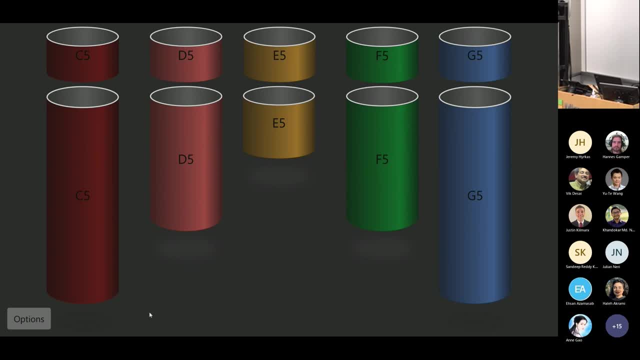 Was that mostly self-reported, like ease of use and fatigue? Yeah, It was self-reported. qualitative measures as well as more quantitative results from the NASA TLX. I dropped my wallet, Yvonne found it and my credit card is just here on the floor. 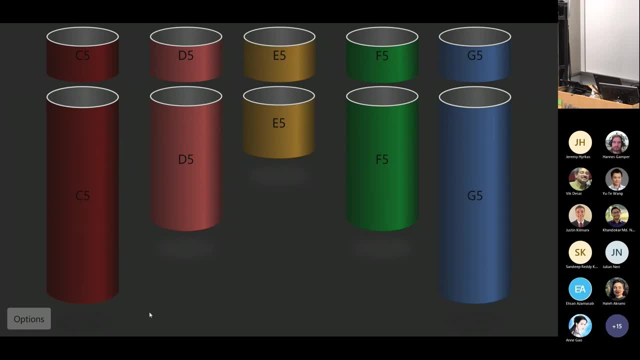 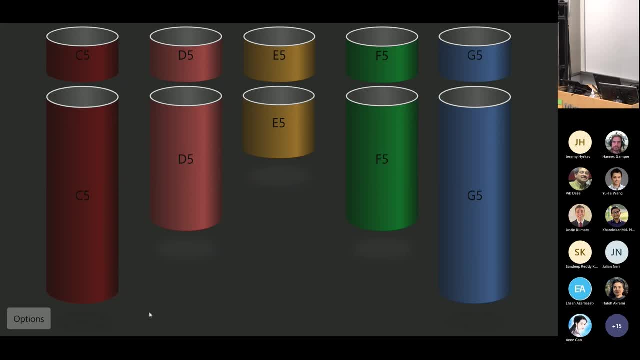 But what we're using now the demo is EEG. What you're using here in the demo is EEG. What I am currently using is actually IMU. Okay, What other modalities did you have? So we had photophlesismography. 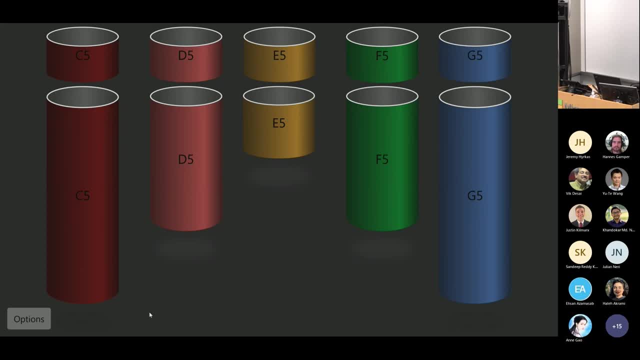 which is the blood flow. and for everyone who might not be familiar with the sensor, this is what you have in Fitbit or other smartwatches that senses your heart rate. It turns out to be on the Muson as well. Do you have any chart or comparison? 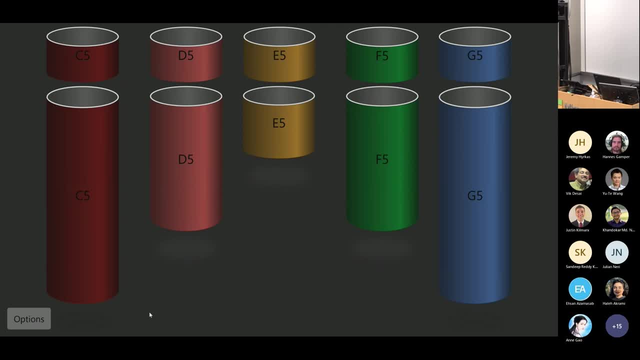 on the accuracies of those modalities. Yes, I was planning to have a comparison on that but unfortunately it didn't make it to this one. I can say that it was almost slightly above chance for photophlesismography alone. 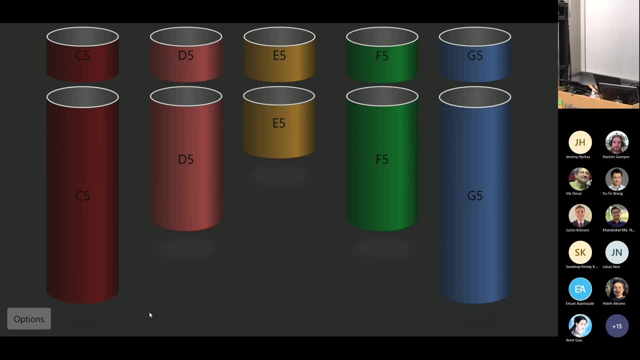 EEG was above chance but not particularly useful for all gestures besides blink and a couple others, because that's also one of the interesting variance points: It's raised by sensor and by gesture At the same time because, for example, ones that generate signals closer to the eyes. 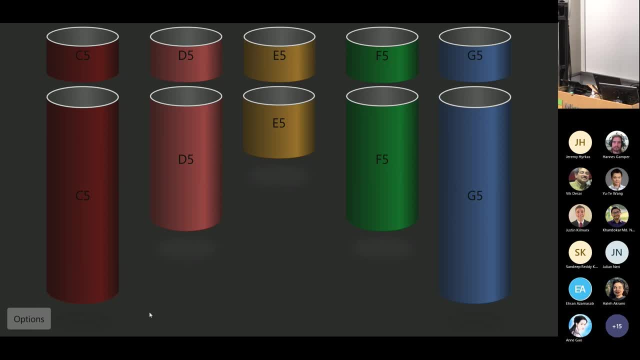 gets much more visible signals on the Muse EEG, because ideally we would have EEG or EMG sensors at the bottom of the eyes, as we can typically have with VR headsets, But unfortunately in this case we only got it from the back of the ears and the forehead. 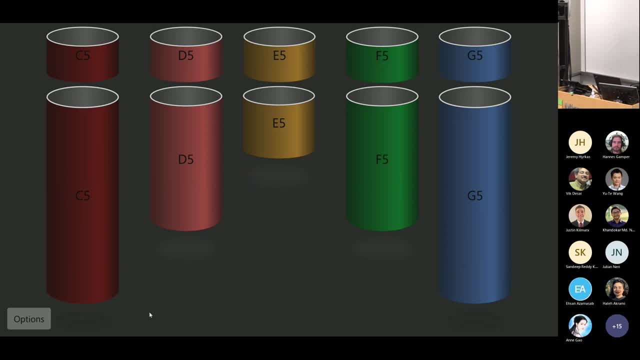 Any more questions Online? I missed that question online, Oh yeah. Oh yeah, Hans was asking about whether it's possible to sense gestures like continuous gestures as opposed to discrete. Yeah, We currently focused on discrete ones. We haven't really tested continuous ones in this study. 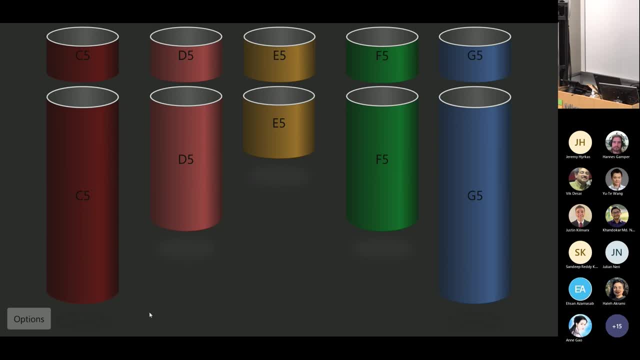 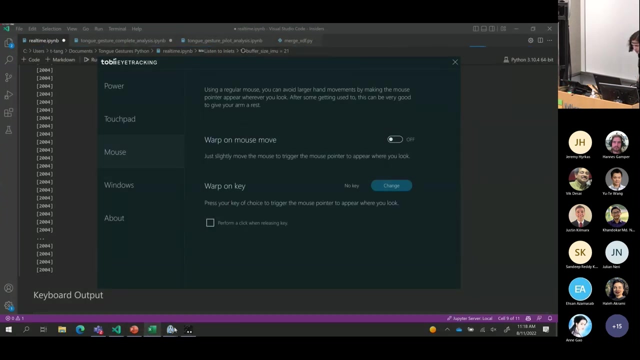 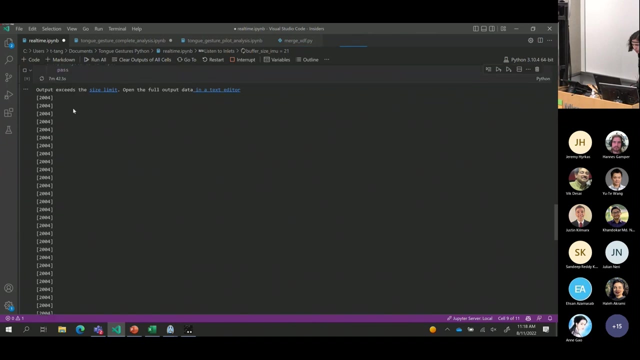 I think it could work, but would require a different model and trial structure is my prediction. Do you have any questions? If there are no questions about the demo, I can continue with the future work for this project. Okay, All right, Let's stop this before I press the spacebar during my presentation. 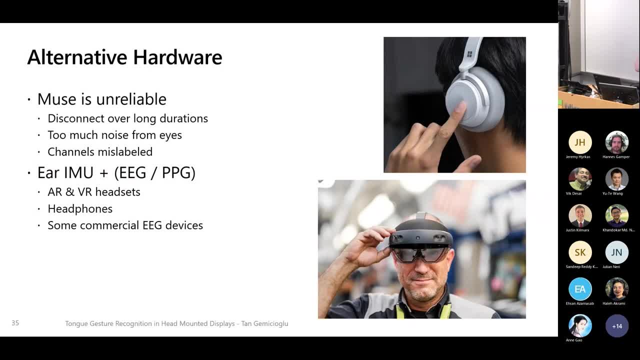 From here on. obviously, I wanted to point out that there's a lot of things that we can do. I wanted to point out that the Muse is not a good sensor for anyone interested in continuing in this space. It's currently disconnects over long durations. 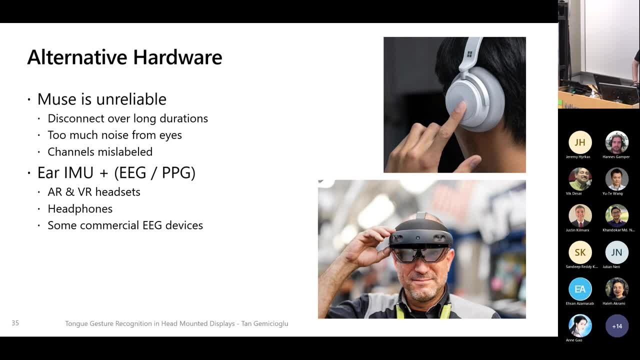 the channels aren't labeled correctly and there is a lot of noise from the eyes when you have sensors on the forehead. In contrast to that, we are hopeful that the IMU behind the ear, as we had with the Muse, and also potentially EEG from the ear. 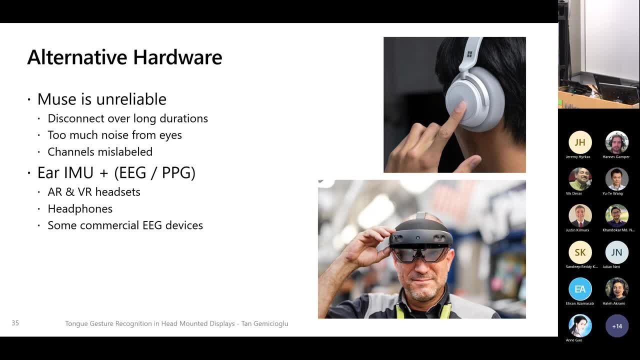 or similar areas could be really useful. We could actually find this to work well with AR and VR headsets, headphones and some commercial EEG devices. The usefulness of photoplethismography is still somewhat uncertain, but it did manage to benefit in. 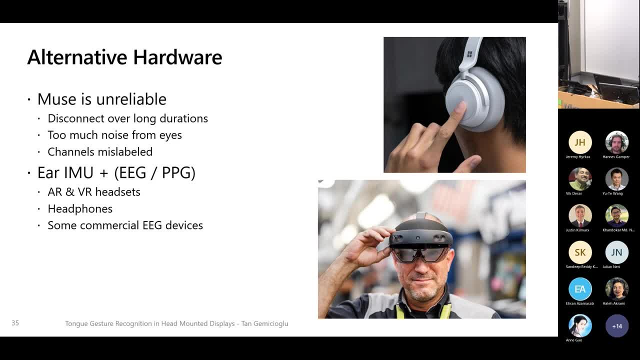 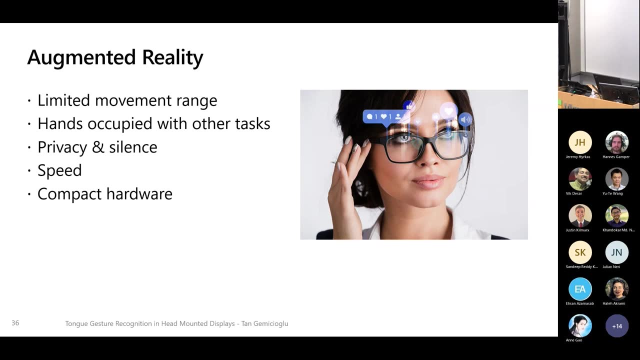 the few multimodal recognizer attempts that I had done, where IMU plus BPG was able to get better results than IMU alone. I think a lot of the benefits from tongue gestures are really applicable to augmented reality scenarios. There's a lot of room to investigate in that area due to the limited movement range. 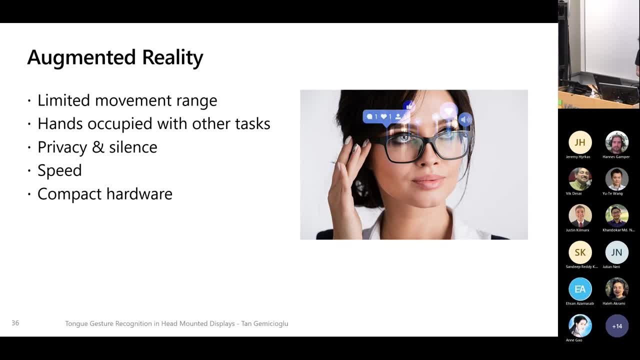 for example, being in a public space or operating under tools Where hands-free interaction is really a necessity. This is also where privacy and silence are really important. Voice recognition is not applicable when you're in a noisy environment or in a space where you need to be silent. 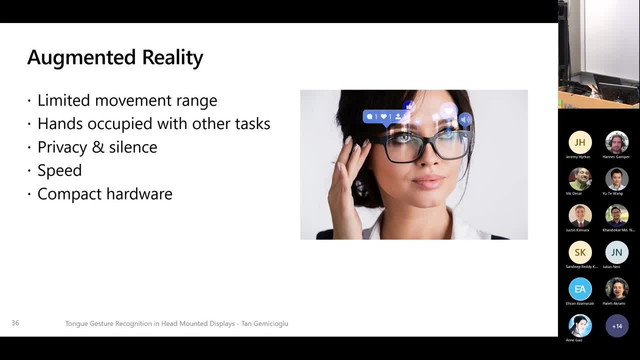 Also being in a public space, you would require a gesture that is more private than, for example, the typical interactions on smart glasses. Also, this is where speed plays an important part, As for people who use augmented reality glasses in their workspace. 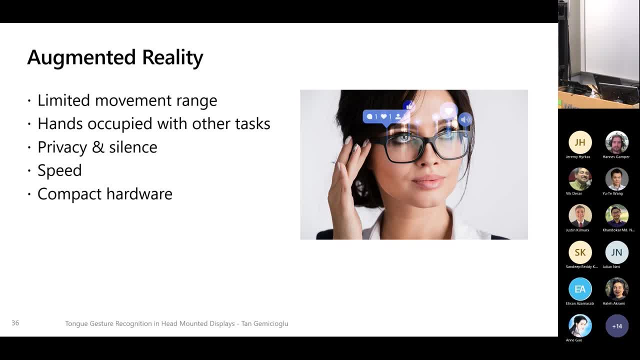 it is really useful to have something that they can interact with quickly, versus delays in, for example, gaze-involved interactions Due to what we saw with the IMU. it would actually also make the hardware a lot more compact compared to, for example, eye trackers. 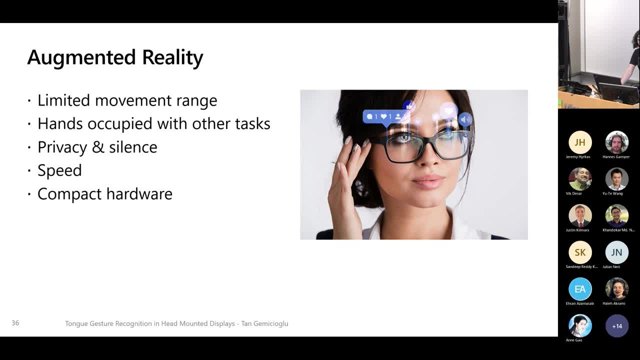 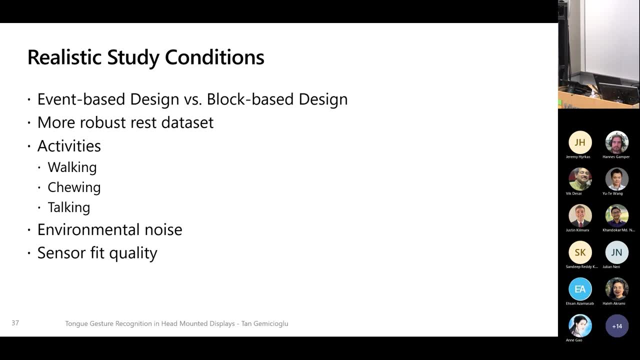 You know, using just an IMU or EEG. As some people have pointed out in previous iterations of this, and as we've seen, this could benefit a lot from more realistic study conditions, While the current work explored a lot of what sensors are useful and what gestures are meaningful. 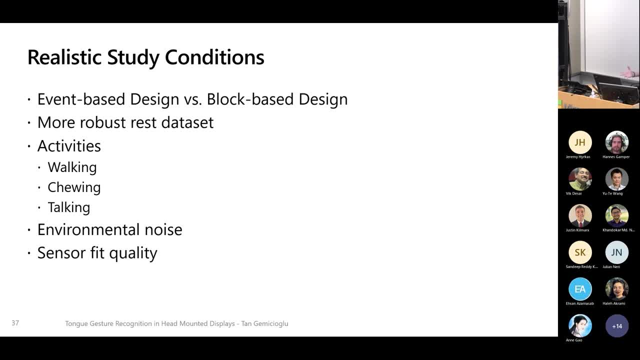 for a real-time recognizer. a more event-based design where we put gestures in between other tasks and rest sessions would help a lot. Such a data set would also help us build a more robust understanding of the rest condition, And we thought that this could benefit from activities such as walking. 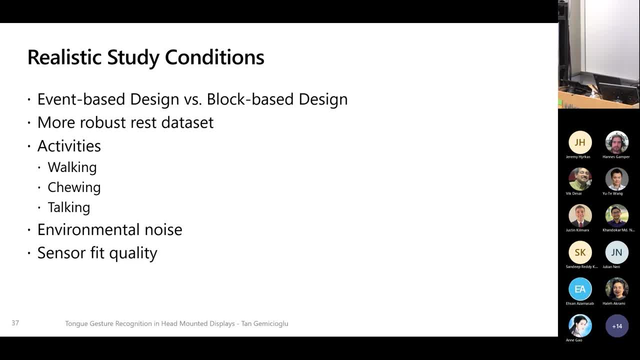 chewing or talking, where the tongue would be engaged but should not be classified as a gesture, And obviously this also is subject to environmental noise and some issues in the sensor fit quality where, due to movement, it might decay over time. 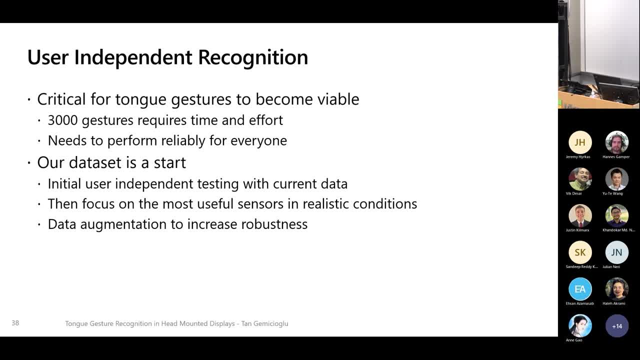 For tongue esters to become viable in use cases in augmented reality or other products. there's still a great need for user-independent models, because collecting 3,000 ester dataset for each participant is very time and effort requiring and we also needed to perform reliably for 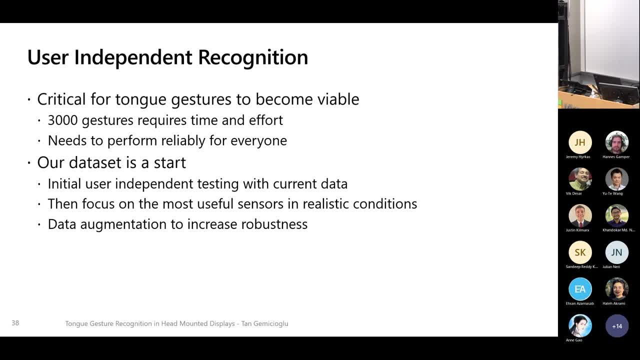 everyone to be able to reach that stage. This dataset, I believe, is a start to getting there. So far I've only done basic tests combining different data from users and, while some sensors slightly translate, this also is with limited accuracy currently. 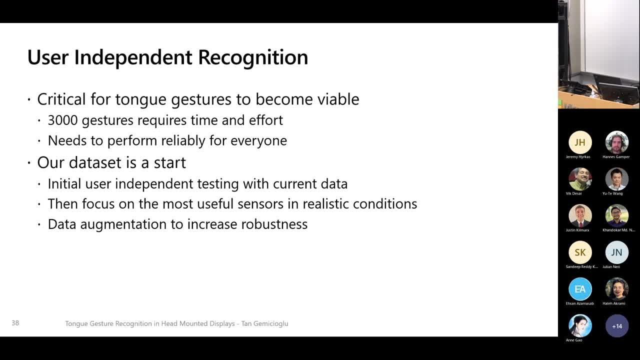 Then I think there should be a focus on the sensors that are most useful in these realistic conditions, and then data augmentation would help a lot in building a dataset that does not require a large amount of gestures from each participant, where, for example, a user-adaptive model could be attempted, even if 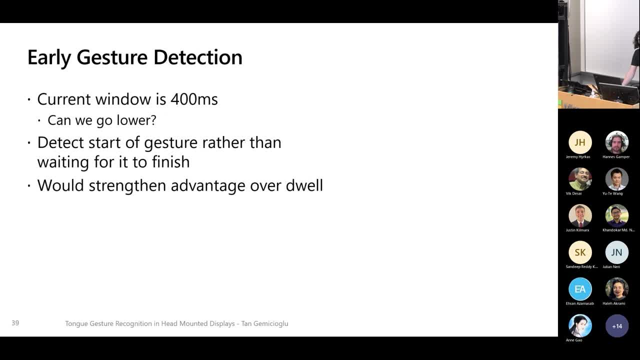 user-independent, does not become possible. We also are interested in how early gesture detection might help, because our current window was about 400 milliseconds, but we believe that it could even be reduced further with the current model, but we could also potentially change it to detect. 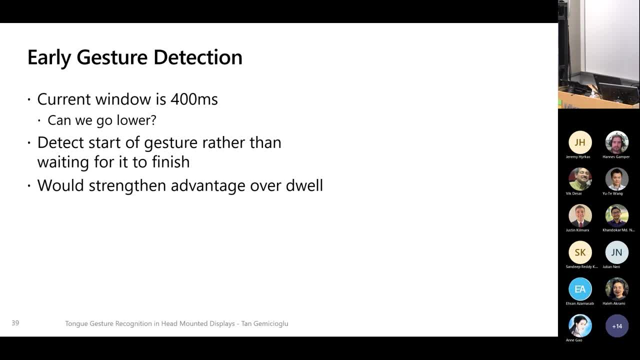 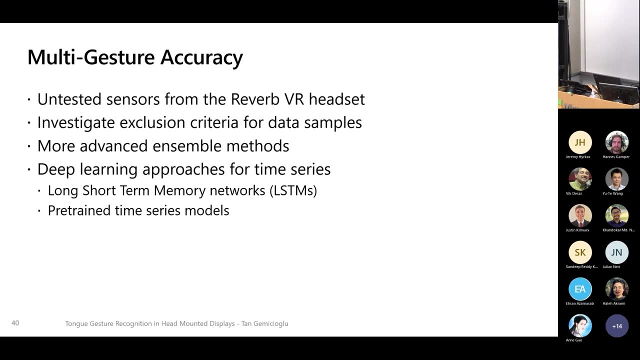 the start of the gesture rather than waiting for it to be totally finished. This would also strengthen the advantage over dwell and allow the tongue gesture to provide more information. Finally, there's a lot of room for improvement in the multi-gesture accuracy. There's still many sensors from. 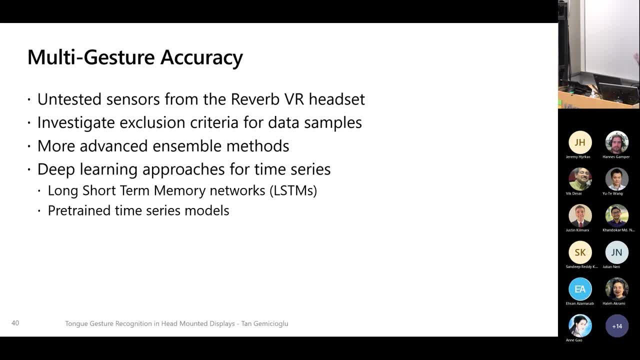 the Reverb VR headset that haven't been tested due to some hardware difficulties we had earlier in the studies. We want to develop the exclusion criteria for the samples further, as this would help determine when there are meaningful gestures and when the sample is corrupted by. 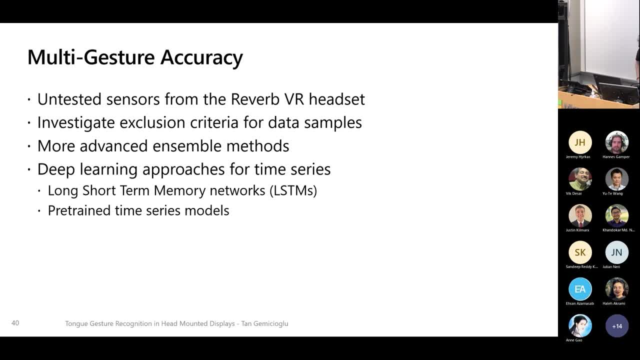 for example, a blink or another signal. There are some other ensemble methods to try that could easily be combined with random forest and have been demonstrated to help with multimodal, multi-modal and multi-modal. However, there's a lot of room for improvement in the multi-modal classification problems and, due to the data set size, there's also room to do deep learning methods that make use of the time series property of the data, such a long short-term memory networks. 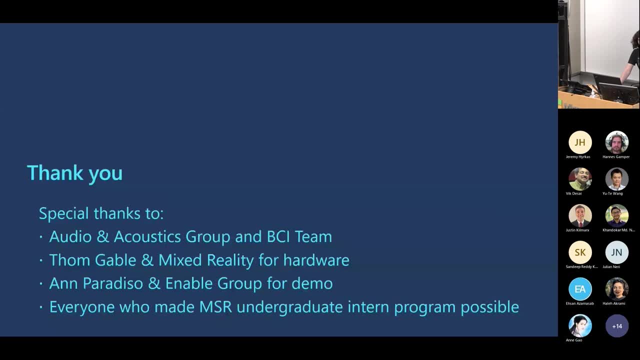 I would like to thank the audio and acoustics group and the BCI team at MSR for all of the mentorship and feedback throughout my internship. Tom Gable and the Mixed Reality team for providing us with hardware and advice. Ann Paradiso and the Enable group for helping us set up this demonstration. 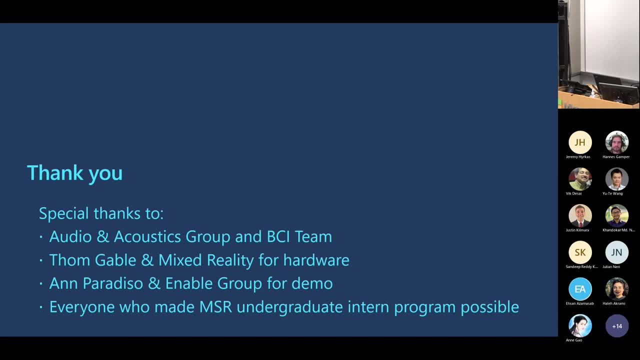 and everyone who made the MSR undergraduate intern program possible for giving me the opportunity to be here- Really amazing. Thank you so much, Tan. Do we have any questions? Did you have any questions from the audience? One already. Hannes, I saw your question. 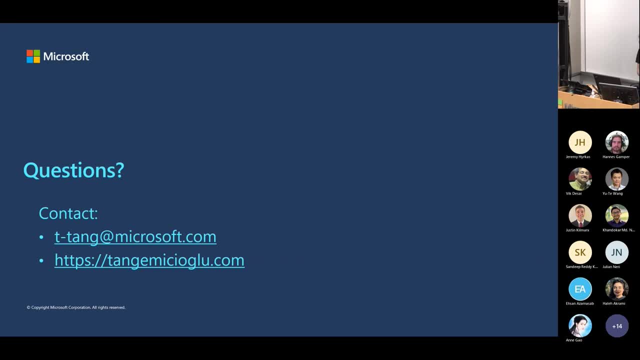 You asked: do you have a sense for how much involuntary tongue movement was present during rest periods? That's a great question. That's one of the unfortunate things about the guess shows being so private in that it's not really possible to judge. Sometimes there was actually head movements by the participants. 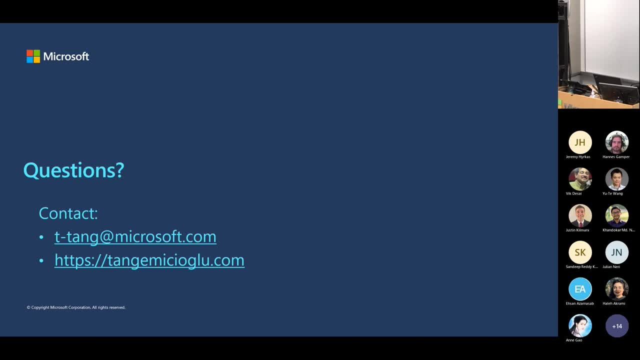 which affected the signals during rest periods? rest periods: sometimes participants talked during rest periods and there were similar issues in many of the rest sessions with the current data set. Thank you, Dimitra. I'll ask the question. So you grouped these time gestures into two factors. one was accessibility. you were looking 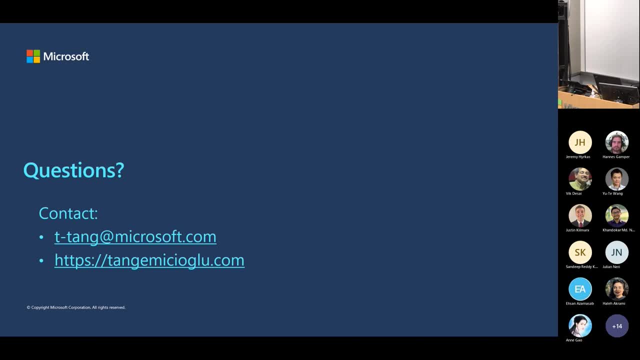 for time gestures, better for accessibility. and the other one was: what was it? the strength of the signal, recognizability, right? There may be one more factor you may be interested in that would be reliability. So I think you collected 300 repetitions per time gesture and it may be worth looking. 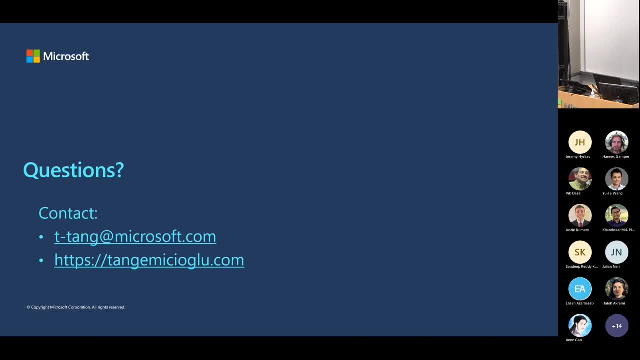 which one are those gestures that have the less variability when you do the repetitions. Maybe you need only one or two to train the model. maybe you need 20 to train the model, versus needing all of them. Yeah, You need all of the 300 to make it robust and reliable. 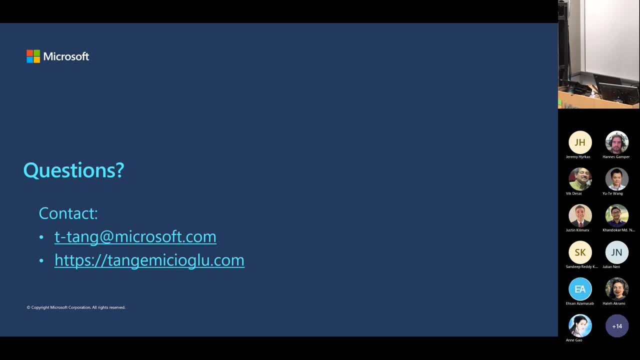 Yeah, thank you for the idea. The current comparisons were across all the gestures, but I can see how that would differ across different gestures. That's interesting, Which may make it easier to calibrate the system. maybe in the future you only need. 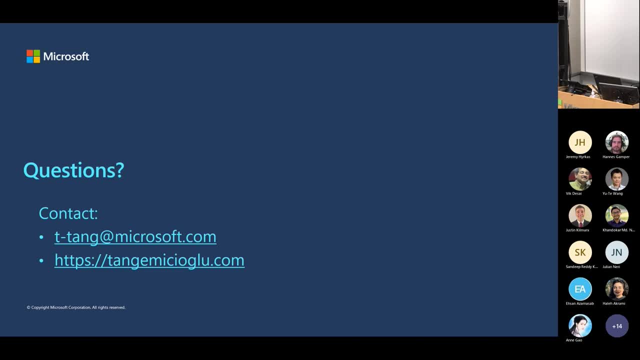 a few seconds to calibrate, rather than right, Any questions from our virtual attendees. Last chance for questions in the crowd. Okay, well, join me in thanking Tan for the wonderful presentation. Wow, Congrats, Thank you, Thank you. 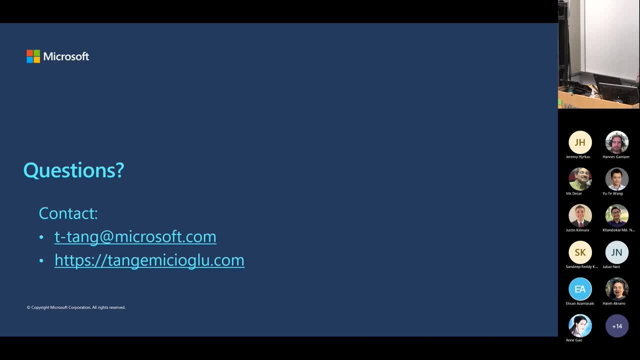